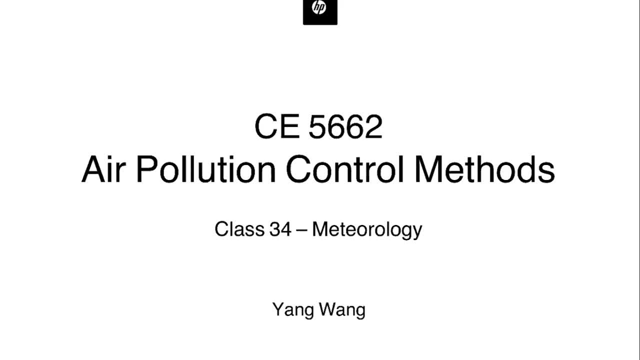 Which is about the meteorology. Okay, so some of you may wonder: why should we be interested in this right? So we spent most of the time talking about the air pollutants. for example, particularly matter the Sulphur dioxide, nitrogen oxygen. 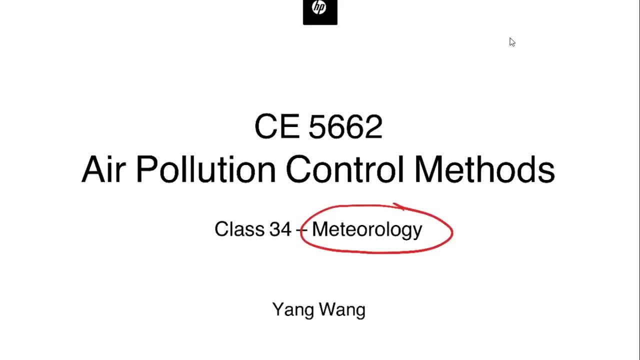 oxides, VOCs and so on. right, So those are mainly talking about the emission of the air pollutants, But the transport of the air pollutant is also very important, mainly because if these air pollutants don't transport, if they just stay where they're being generated, 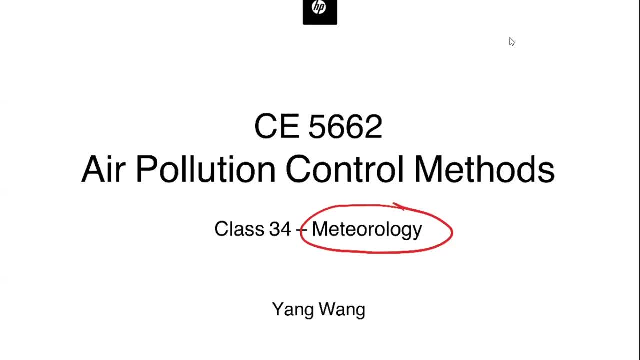 then we won't have any of the air pollution problems. It's mainly because they're going to disperse and also they're going to get transported to different locations, And it's during this process that's causing health hazards to the human right. 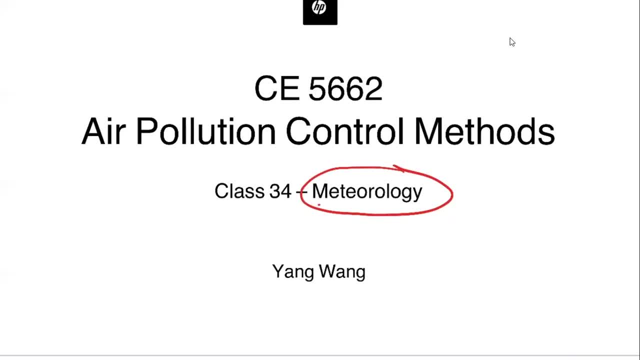 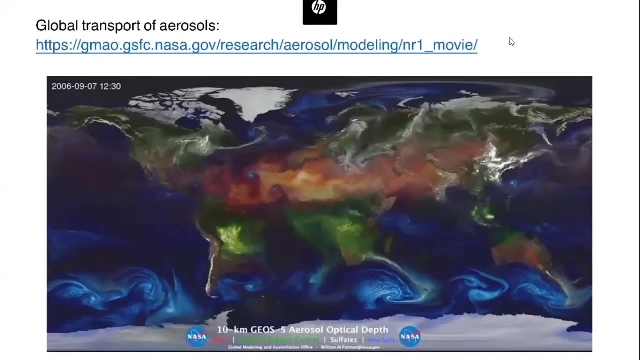 So that's why we're very interested. We have to pay attention to the meteorology, which involves the transport of the air pollutants through the winds right. So I would say the wind direction, the global wind direction, the wind pattern is going to be the most important content. 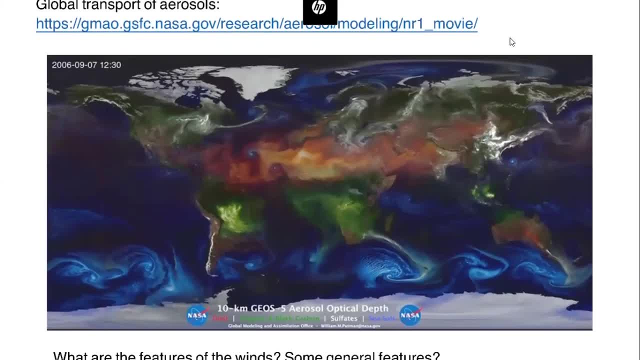 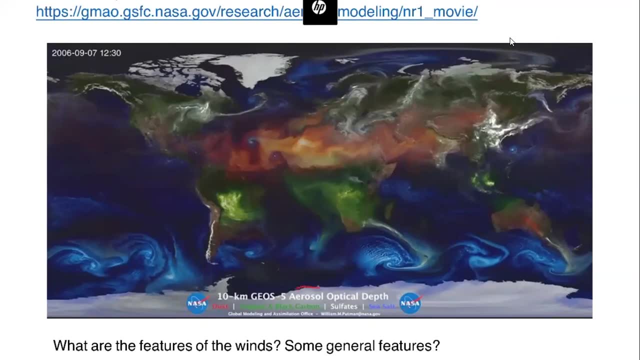 regarding the meteorology, right? So here I'm showing a graph about the global transport of the aerosols. This is showing the aerosol optical depths, So you can just think of this as the concentration of the PM, okay, So basically, this graph is showing how these PM 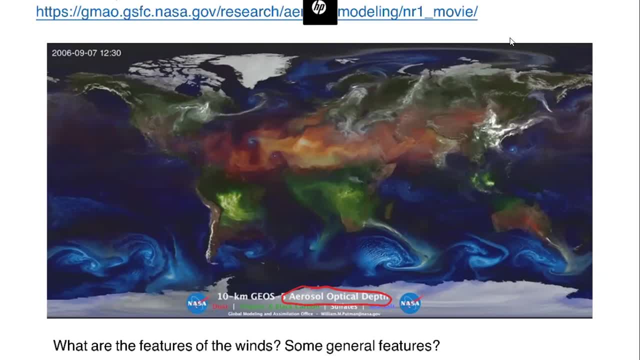 where these particular matter moves in a global pattern and also have a video to show this process. So basically, these PM will move because of the wind right And based on the movement of the PM, you can try to basically try to see some. 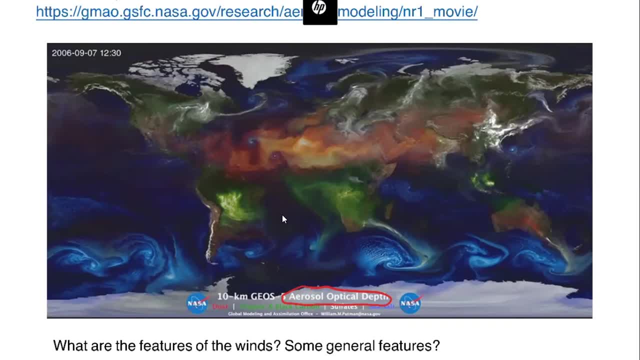 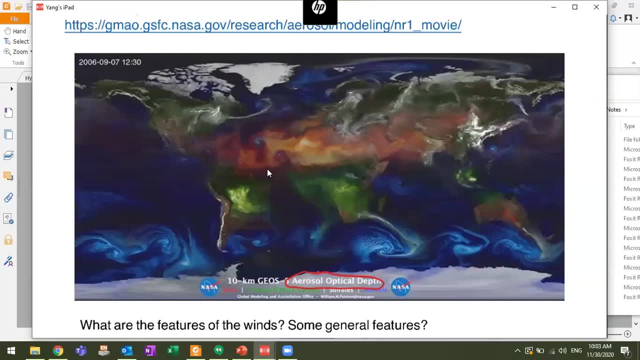 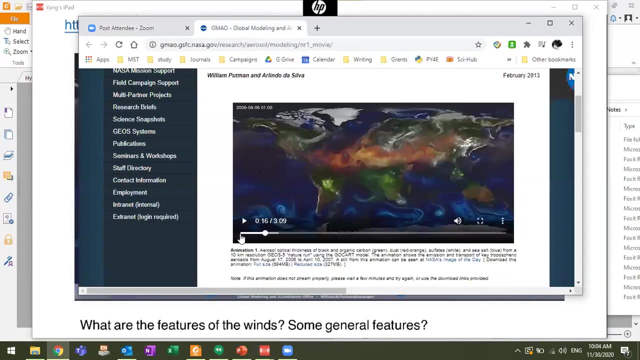 answer some questions regarding what are the features of the global wind patterns. So are there some general features at all in terms of the transport for these, either the particular matter or the wind? So I'm going to show this video And also this is what's being captured. 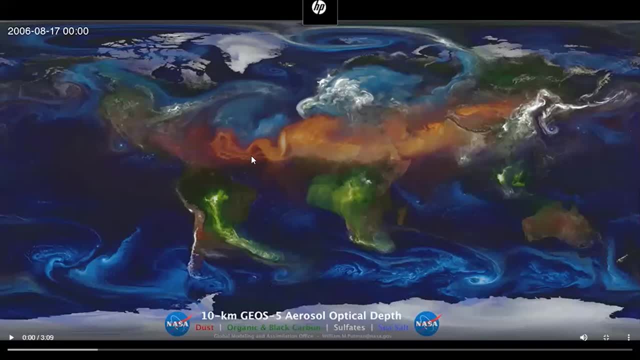 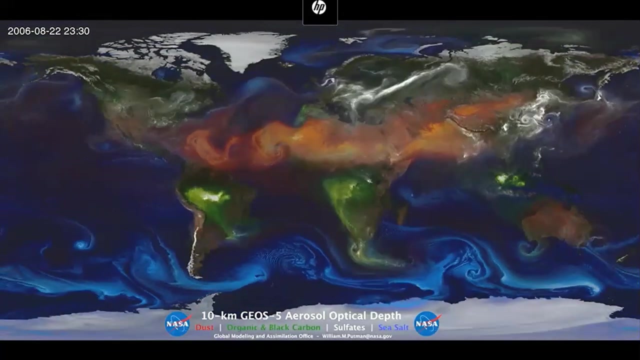 from the NASA satellite. okay, So this is basically a replay of the transport of these different aerosols globally. okay, This happened on 2006.. Okay, so let's try to see whether there are some general patterns. So, if you look at the equator, 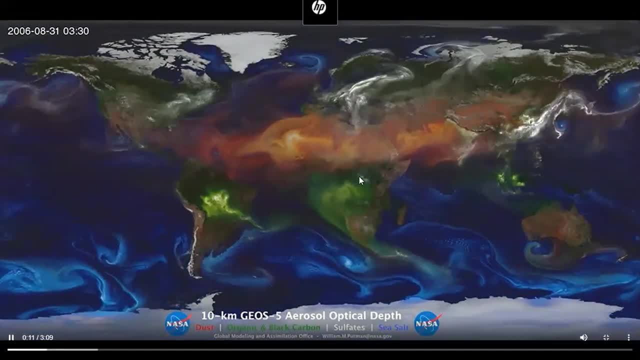 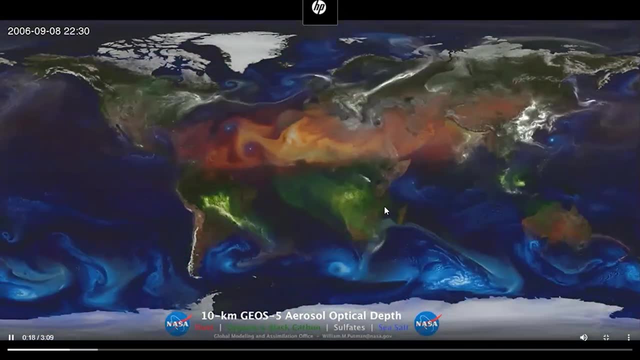 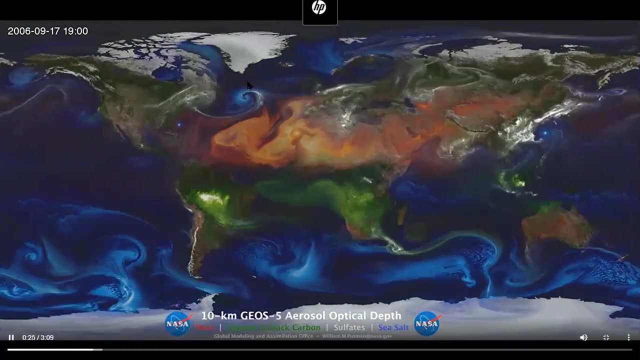 you can see, the aerosols are being moved in a general pattern right, Either from east to west or west to east right, And also there are stronger winds, generally at the mid-latitude or at the Arctic region, Antarctic region. I see the wind here is very fast compared to other locations. 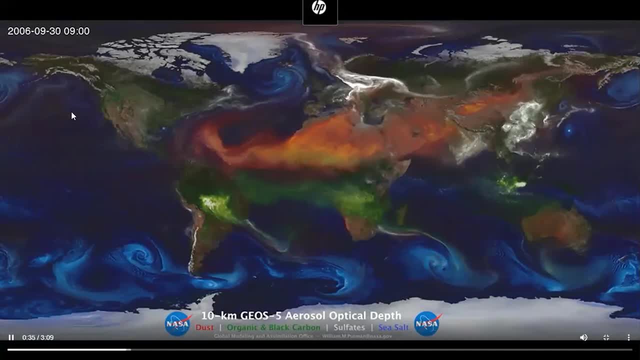 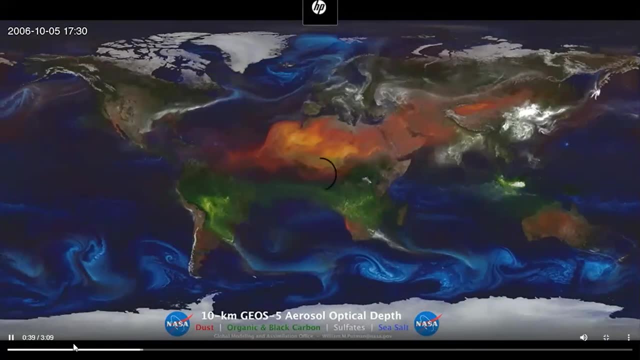 And also in the mid-latitude. you can see, for example. this is US right, So you can see the aerosols are being transported somewhere And although there are some- let's say there are some- swirls of the wind, 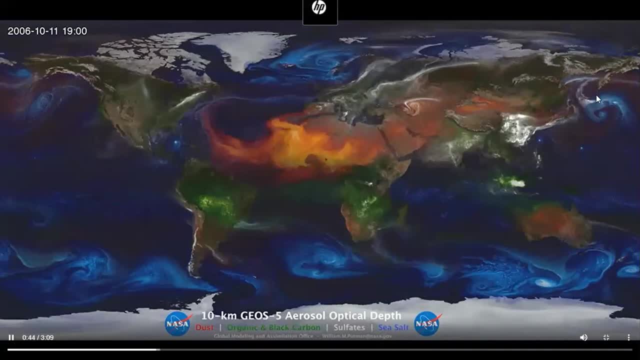 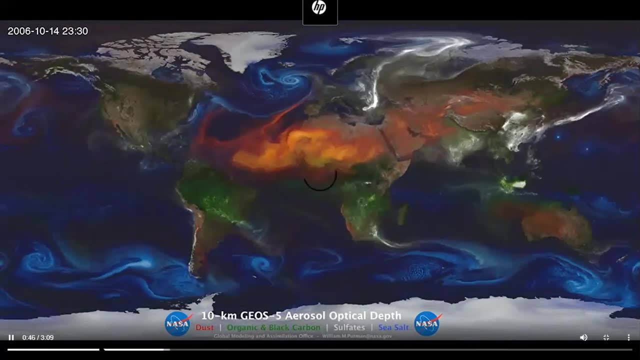 but in general, there's a trend for the transport of the aerosols. okay, I think the internet might be stuck for a little bit, right? So if we just look at this, let's say this is US, right, So this is China. 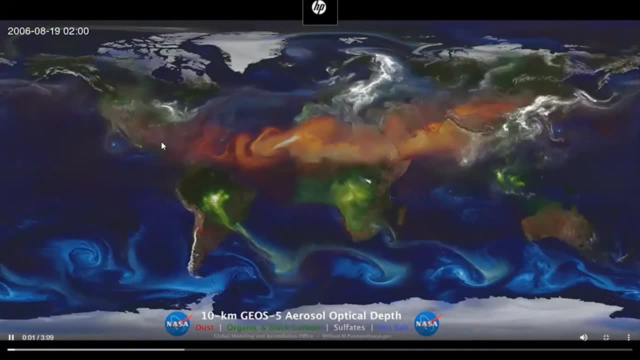 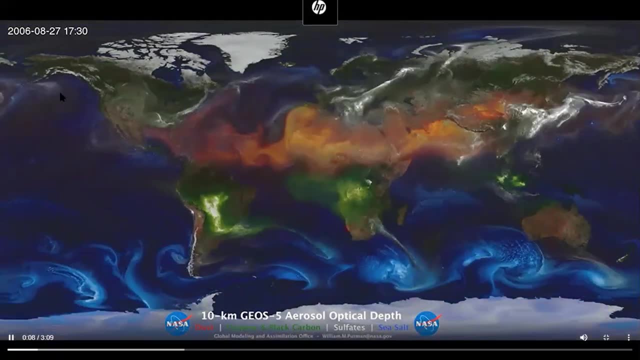 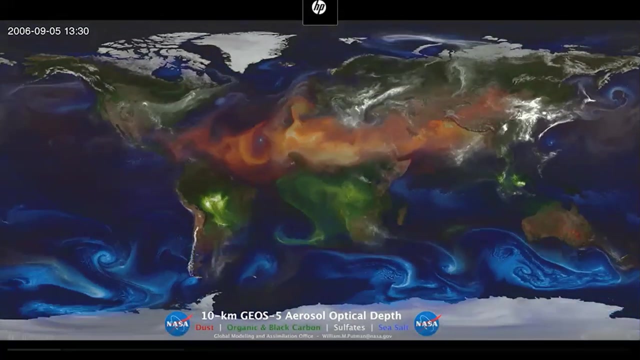 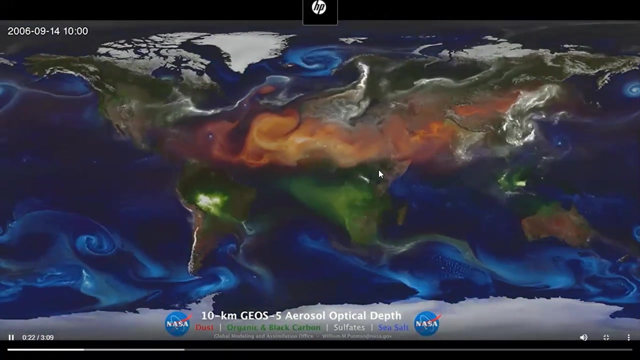 look at the situation from the beginning And also notice the time here. this is day by day, So the wind actually moved pretty fast right. So now if I ask you a question, it's based on this video. here, I mean, which direction is the wind near the Equators? 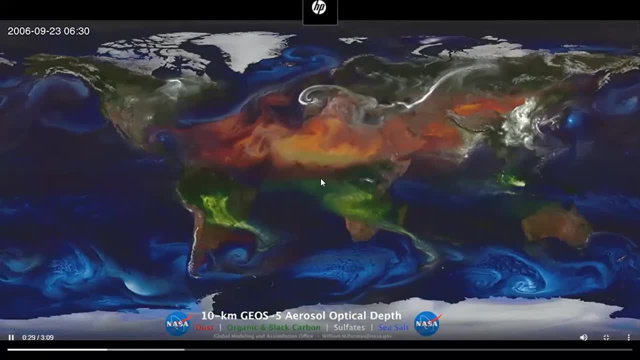 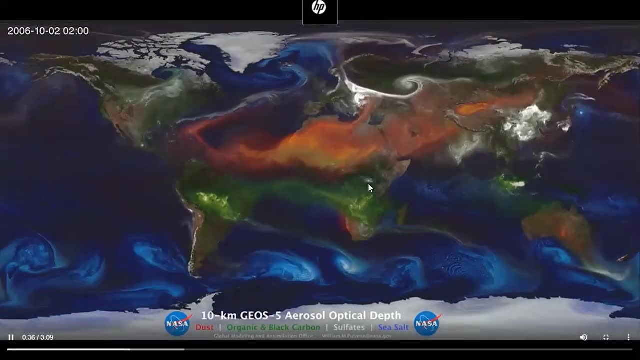 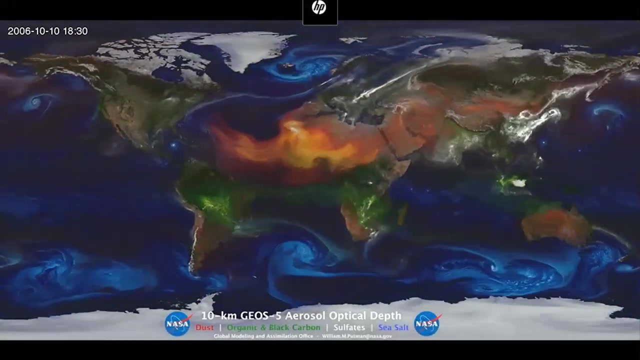 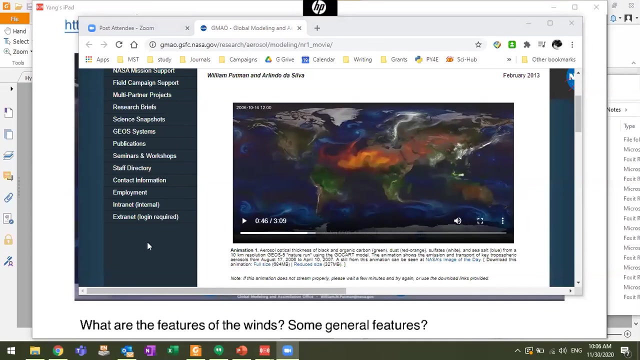 You see, the Equator is basically near the Amazons right, And also near the Sahara Desert right And also somewhere over the Africa region, Right? so if I give a quiz, So what is the direction of the wind near the Equators? 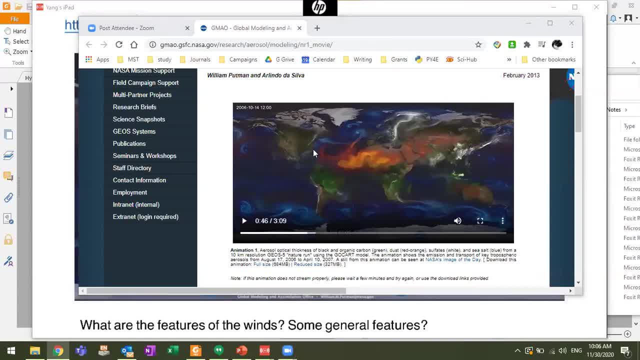 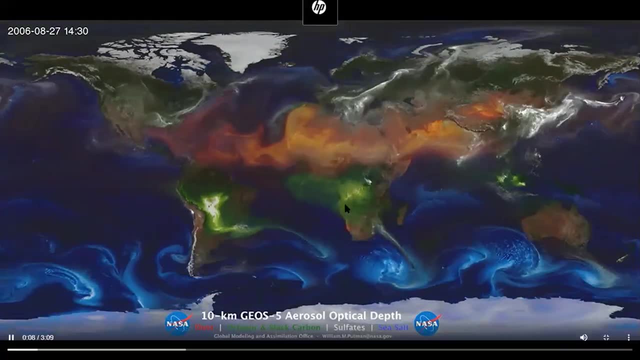 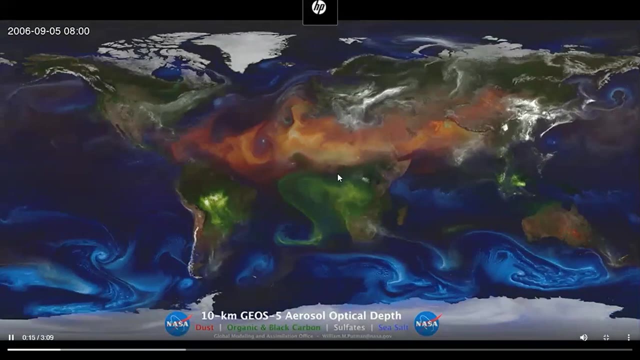 Is it from west to east or is it from east to west? So if I just show this again, I think it's probably easier to just look at the the direction of the wind. So the direction of the wind is going to be from west to east. 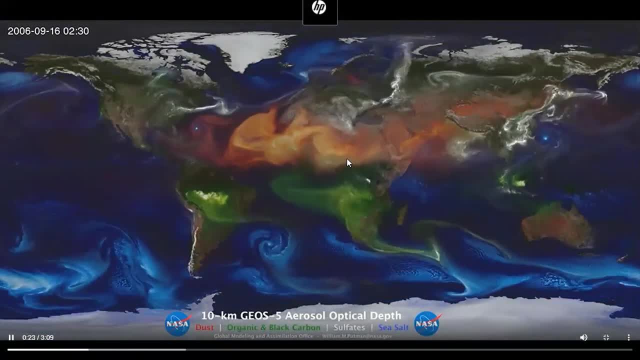 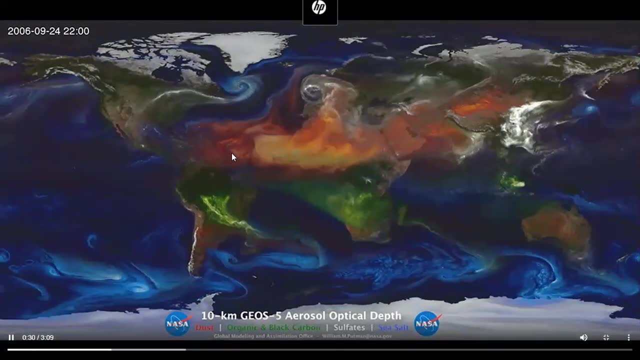 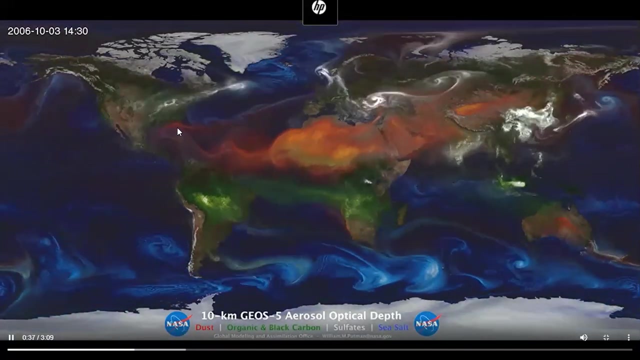 So from west to east, we have a general trend of the dust aerosols, basically the sand that's being generated from the Sahara Desert. right, You see, there's a general trend that these dusts are being transported from the Sahara Desert to the west. 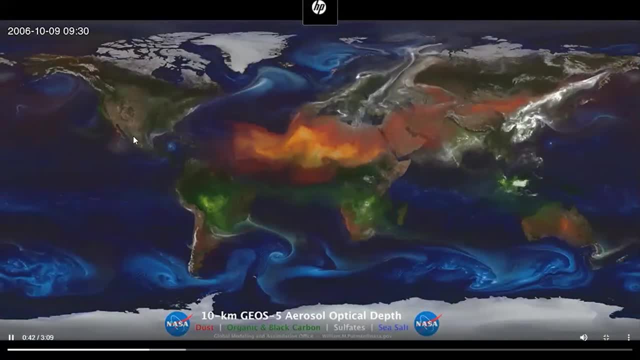 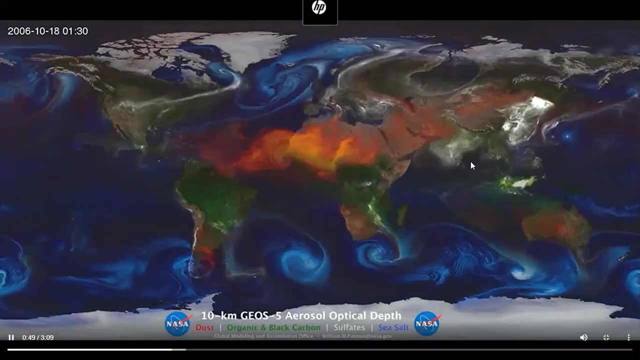 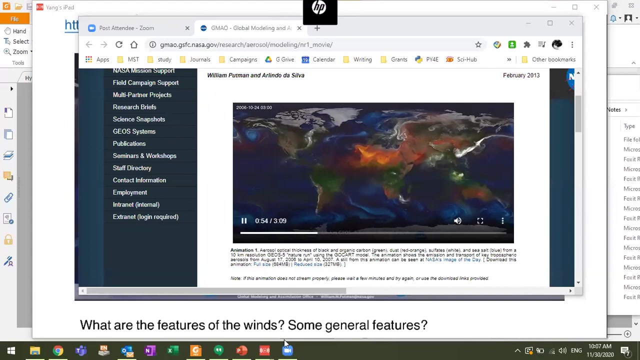 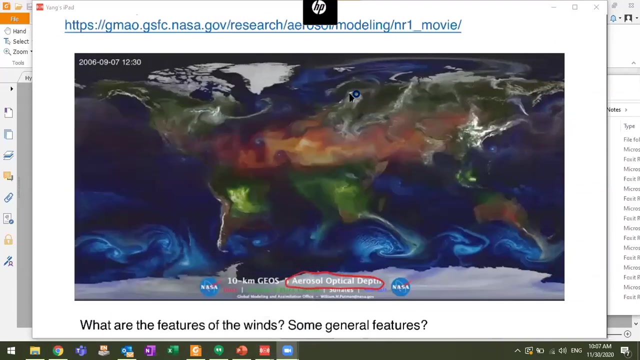 Basically, direction is going to be east to west, right. That's why even North America separate region, Otherwise, these dots are going to flow in this way, right? So now you can see that the correct answer should be. let's see, Okay, So the correct answer should be east to. 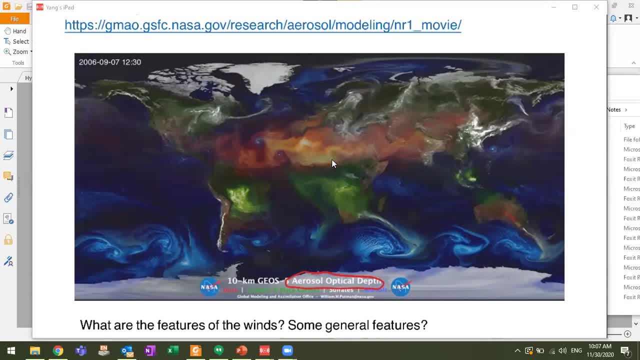 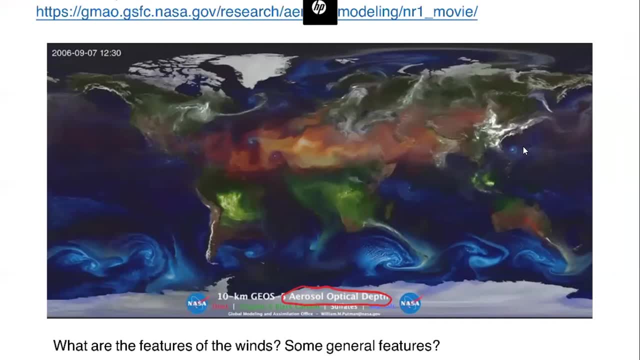 west. Okay, So this should be the direction, or the general direction, of the wind near the equator region. So then you may wonder why this is a case right? So if you further track the features, not only near the equator, we have this general direction of the wind over the mid-latitude. 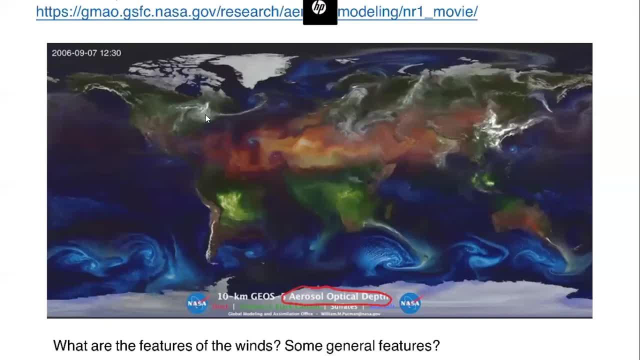 Generally, the wind direction is from the west to east. You see, these aerosols are being generated from here and then getting transported In this direction And further at higher latitude, higher latitudes, for example the Arctic region or the Antarctic region. the wind direction is reversed again, It's from east to west. So 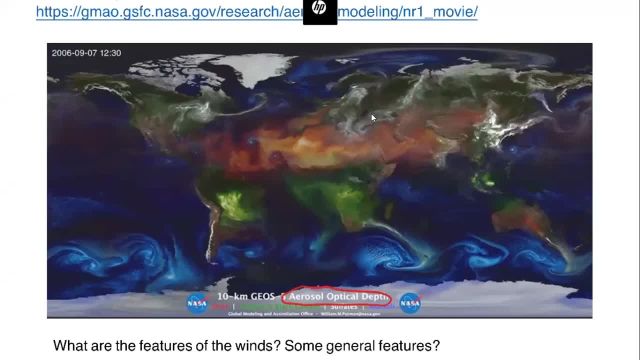 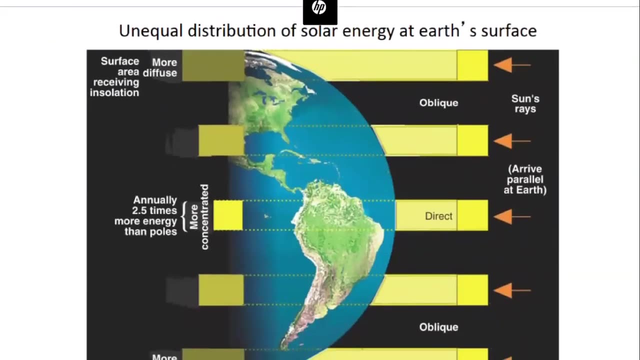 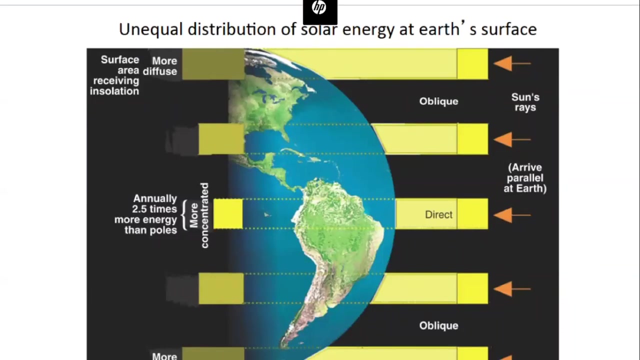 basically, we have this east to west direction, west to east direction. in the mid-latitude and higher latitude, we have east to west again. Okay, So why this is the case? So this have to be something involved regarding the Earth's energy budget, Basically the radiation that we receive from the sun. Okay, So whenever we 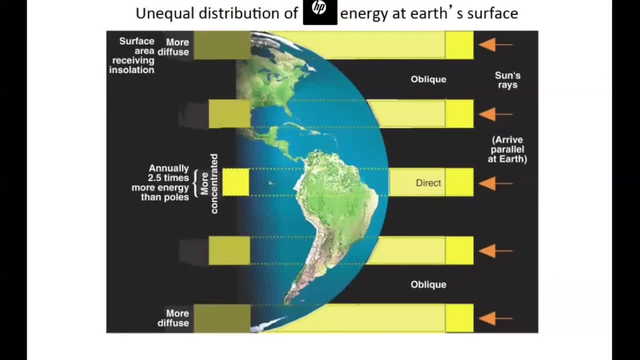 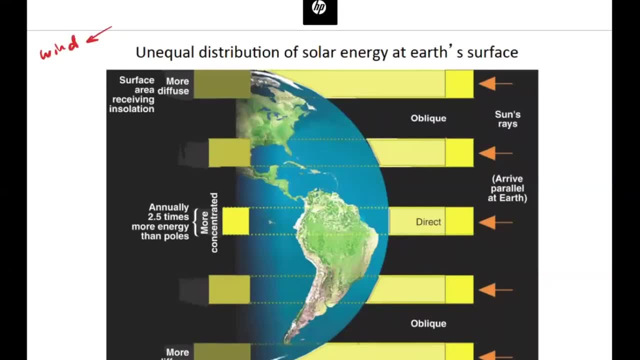 describe the generation of the wind. so the wind is basically caused by the pressure difference, right? So just think about, think about the scenario when you're trying to blow some air from the mouth, right? So if you do that, you're going to feel a wind, right? And that wind is caused by the pressure difference, mainly because 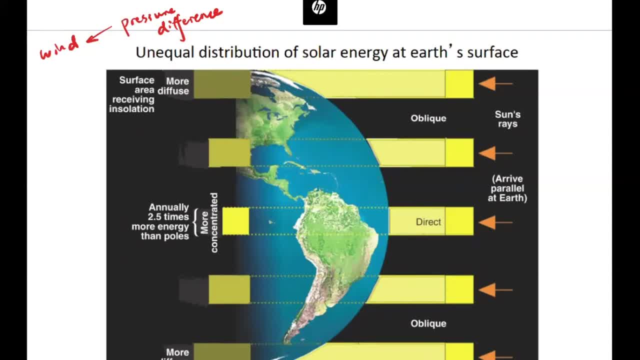 the pressure in your mouth is higher than the ambient pressure. Okay, And it's the same, basically, for our Earth as well. right? So the wind on our Earth is caused by this pressure difference, And the Earth doesn't have a mechanism, Right So you know, perrontal air is designed to create a higher pressure, just like we we're trying to blow the air from. 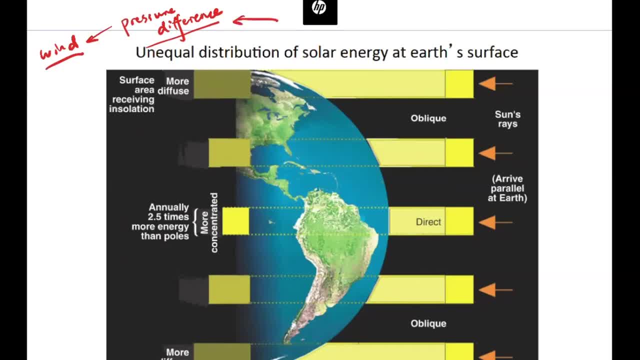 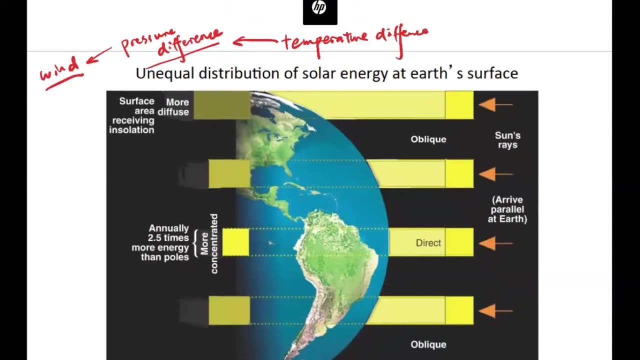 our mouth. So what it does is further use the temperature difference. So, according to the ideal gas law, we know that the higher temperature. if you have a higher temperature, then you're going to have a lower density of the air Right. 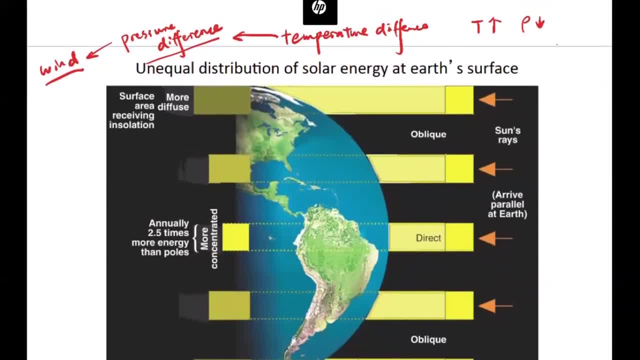 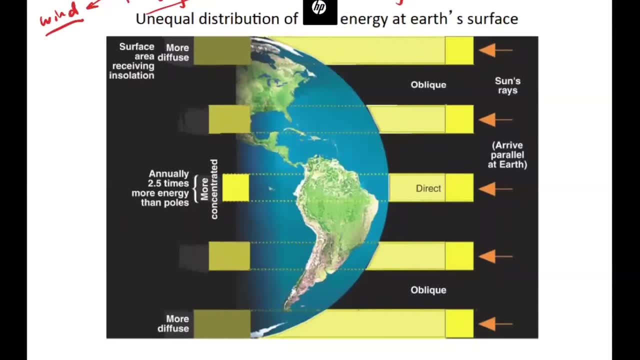 Okay, Right, lower density, then the air is going to try to lift up, right? so basically, if you think about our earth, then we have the warmer regions and also we have the colder regions. like the warmer region is going to be near the equator, mainly because 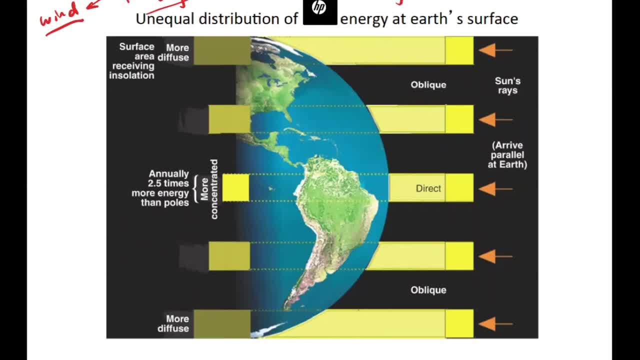 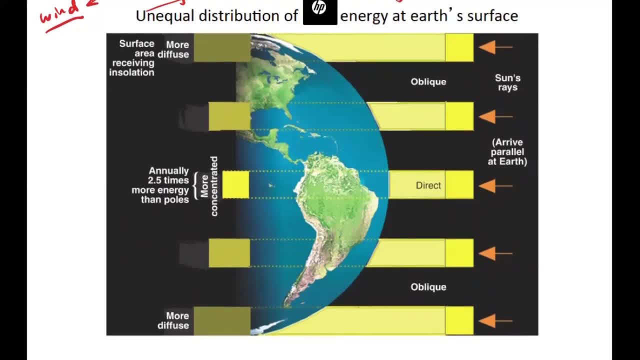 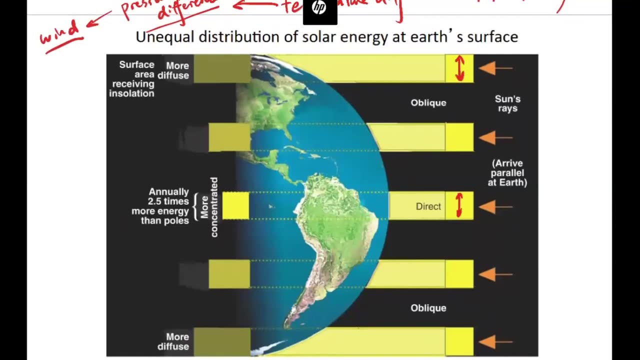 for example, this is a solar radiation, right, because our earth is so small, so all of these radiation are going to be parallel to each other, right? and then, if we think about the energy that's emitted at this location, and the energy that's emitted at this location, so their 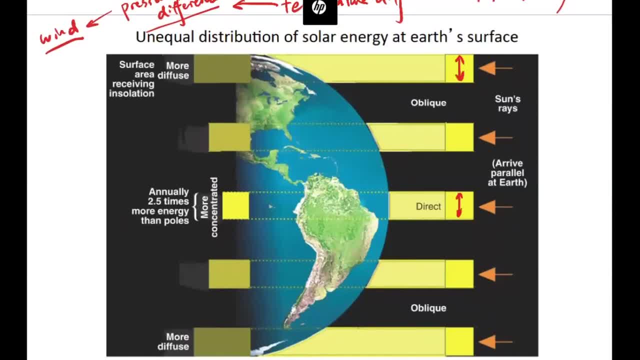 energy, basically, is going to be the same right, so we're going to receive the same amount of energy, which is q over this, over this area here. but because of the higher latitude region, we have this curved structure here. so what that means is we have a larger area. 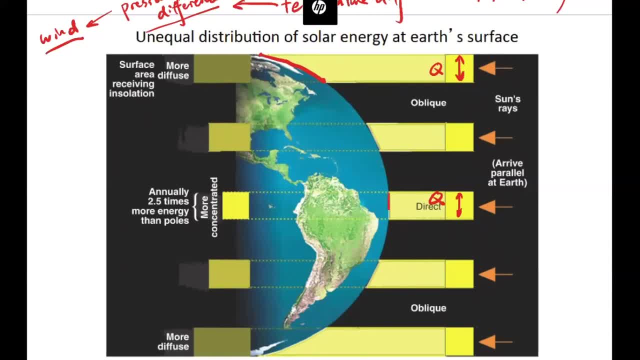 to receive the same amount of energy compared to the equator region. so, basically, the temperature here at the equator is going to be higher compared to the temperature at the higher latitude, mainly because we receive a higher density of the energy from the sun. right? so because? 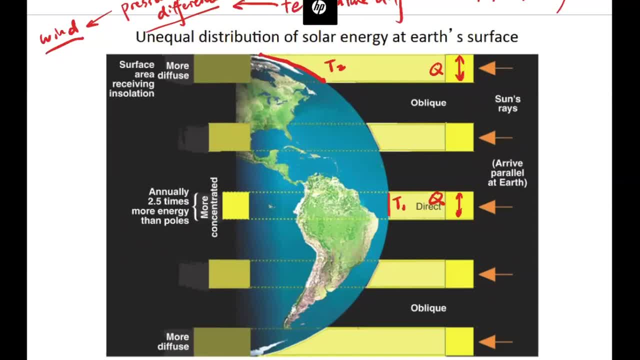 of this temperature difference, the air at the lower latitude, basically at the equator region, are to rise up, while the air at the higher latitude are going to fall down right. so this is based on the ideal gas law. we're going to have this general pattern in terms of the wing right. 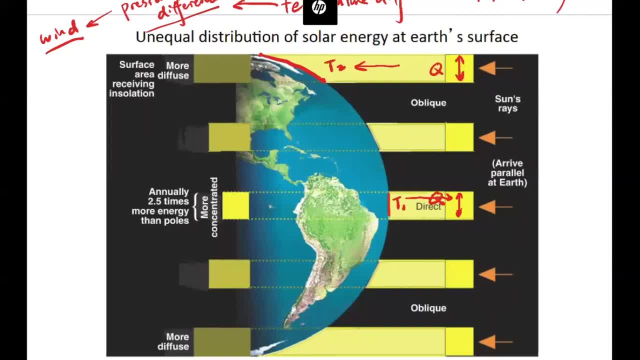 so if the air warm, warm up, or if the air lift up at the equator region, then we're going to have a low pressure. we're going to have a low pressure zone near the equator. so what this also means is that the air are going to flow in this way, right from the south to 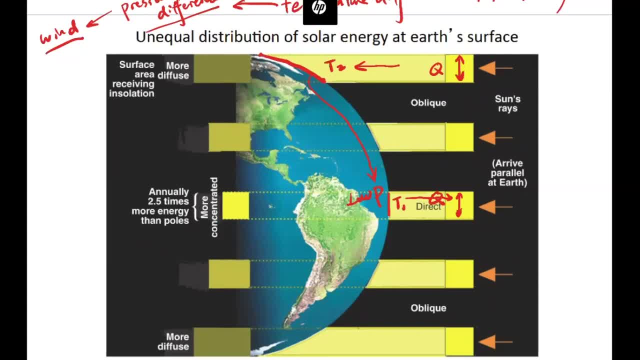 the north, from the north to the south in our northern hemisphere and in terms of the southern hemisphere, that's going to be south to north, right? so basically, we have a low pressure zone which attracts the air from the arctic region or the higher latitude to the equator. 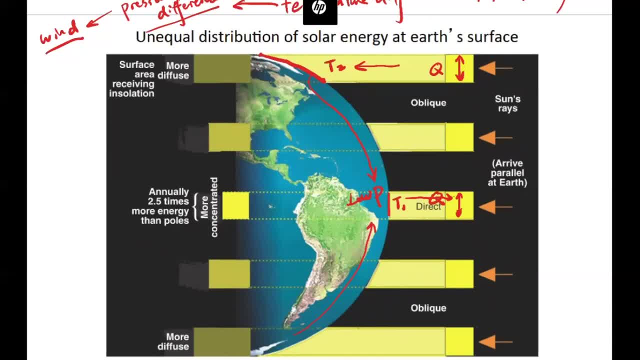 region and, at the same time, higher altitude, higher heights, the air are going to go this way. okay, So this is going to be the general wind pattern on Earth, And this actually applies for a lot of the planets, right? 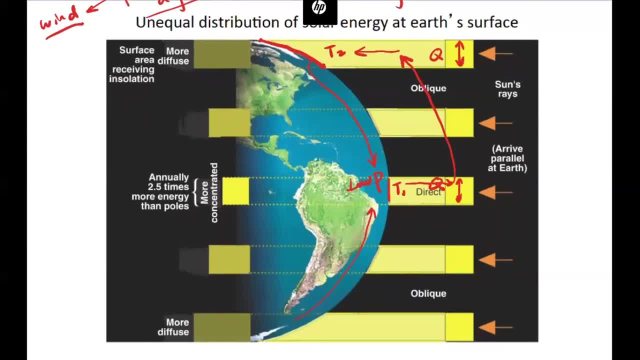 So let's say for typically, for the smaller planet, okay. So if we have think about a small, let's say a billiard ball, okay. So if it's going to be a billiard ball that's receiving the solar radiation, 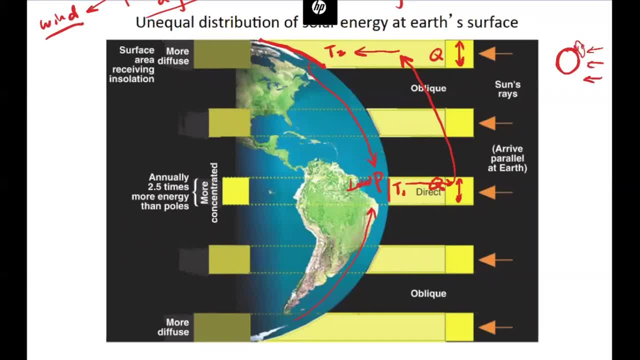 then we're going to have this general recirculation of the air. Okay, so basically, at the ground the air is going to lift up near the equator region and then, at the higher latitude, the air is going to settle down because of the colder air in here. 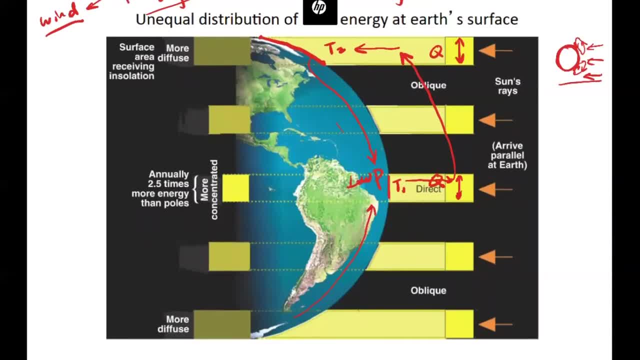 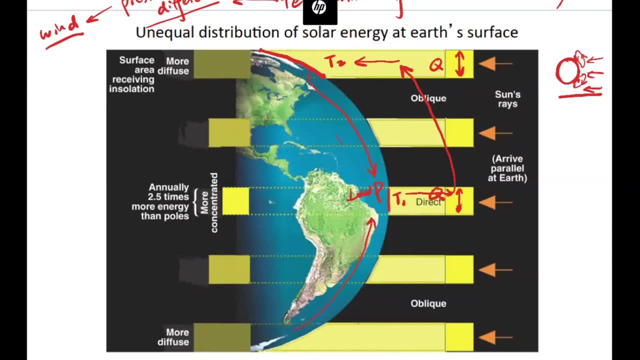 And this is going to be the scenario for a relatively smaller planet or, for example, a billiard ball. okay, But unfortunately, our Earth is not a billiard ball. Our Earth is so large- right, It's so large- that it has to break up. 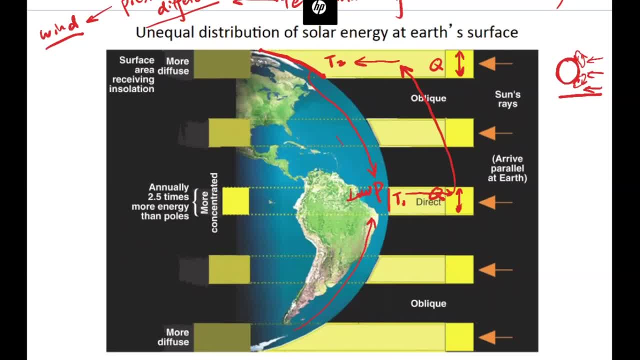 into several recirculation patterns. So what happens is, instead of having this long range of the wind flowing from north to the south right, mainly because this distance is so large, it's broken into several sections. So first, at the higher latitude, 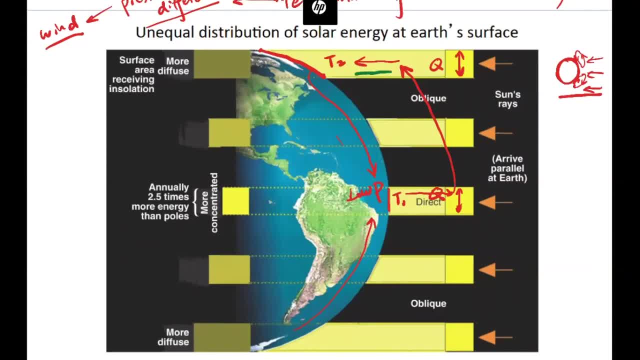 we're still going to have this general pattern where the air is going to settle down At the higher latitude near the Arctic region, And then it's going to go this way, then this way, and then this way. Okay, so it's going to form several cells of the air. 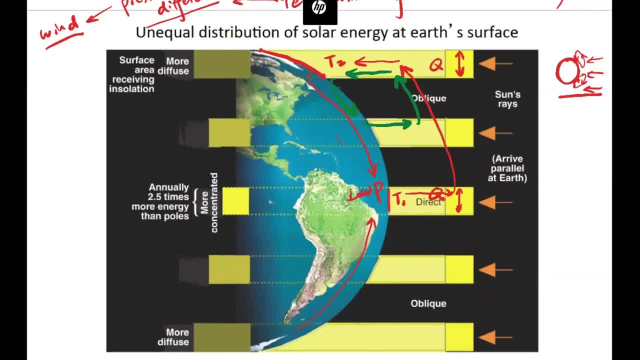 Well, at the equator region you're still going to have this air lifting up and then go this way, settle down And then further. we go this way. So basically, Arctic region and at the equator region you're still having this pattern. that's regulated. 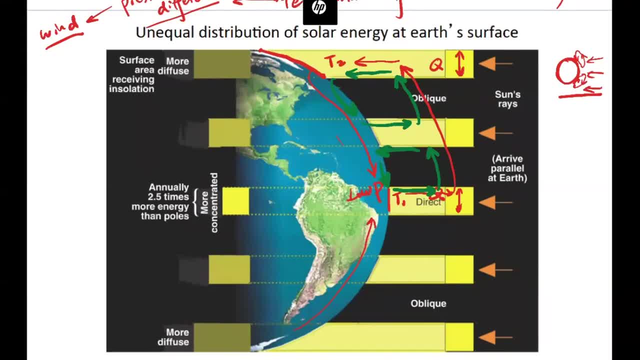 by this, higher temperature air warm up right and lower temperature air settle down, And then it's basically at the mid latitude. we're creating a new cell which has the air circulation like this: Okay, and this is mainly because of the air movement direction or the wind. 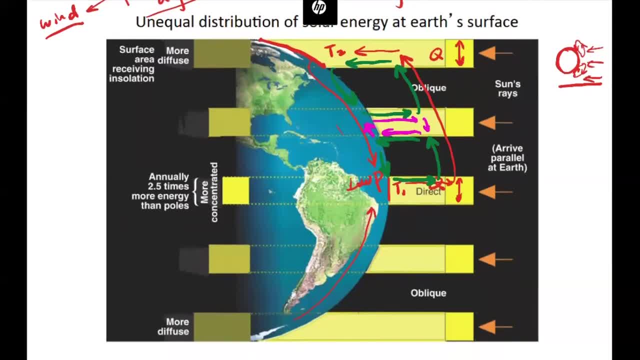 direction at a higher latitude and that lower, lower latitude, lower latitude, that's creating or enforcing this circulation of the air in the mid latitude, where the air is going to go go down further at the lower latitude and then rise up at a little bit higher latitude. 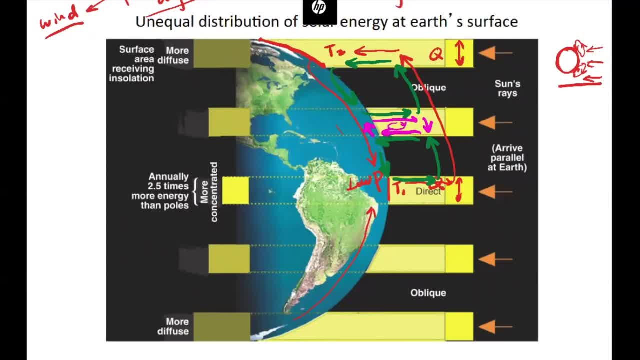 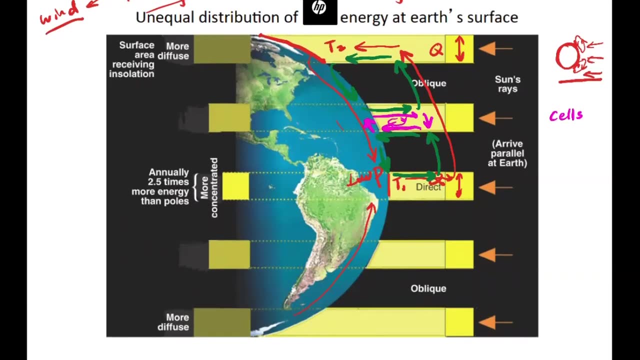 So basically, we're forming another cell in here, Okay, and we generally call these circulations sales, and each cell actually have their own names, Right? So this is a scenario for the northern hands hemisphere, And the same thing is going to happen for the southern hemisphere, where 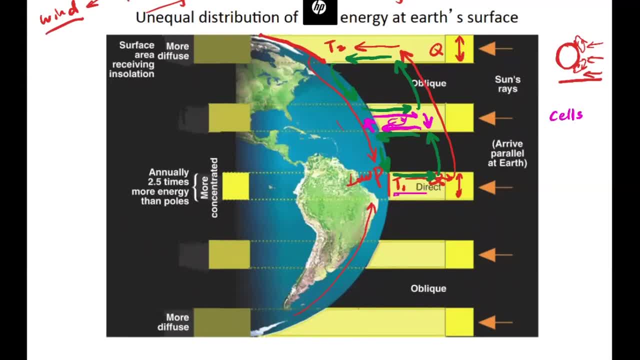 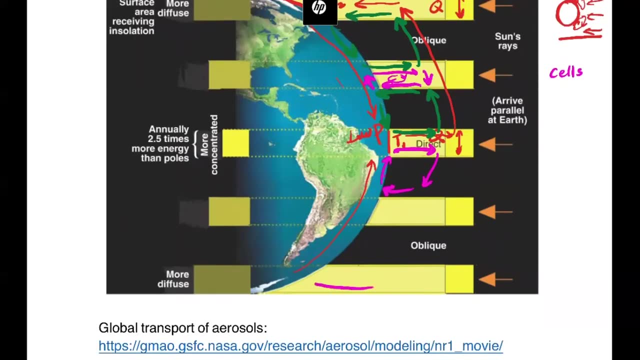 you have this air circulation, Air warming, rising up at the equator region and then go this way, This way, this way, Near the equator region region, and then at the Antarctic region. we have air settling down here, rise up and then go this. 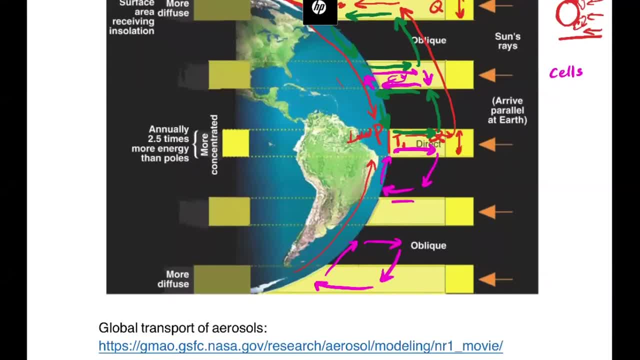 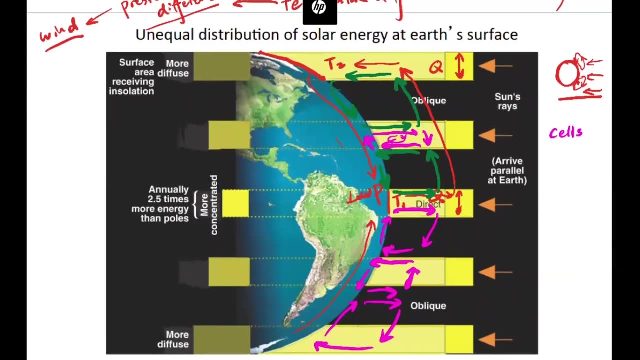 way. So in the middle, in mid-latitude, we're enforcing air recirculation. that goes this way, okay, So theoretically, if our Earth is very small, it's further smaller in terms of its size. then we're going to just have two cells, okay, Just northern hemisphere and southern hemisphere. 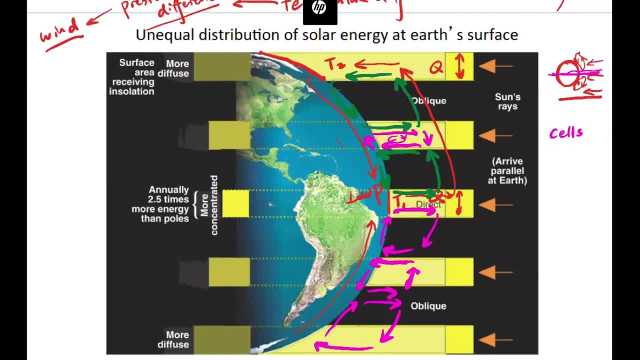 But because the Earth is so large, it cannot maintain this large scale of the air recirculation, so that's why it's broken down into three different cells, right? So number one, number two and number three: okay, The same situation will happen for the southern hemisphere, right. 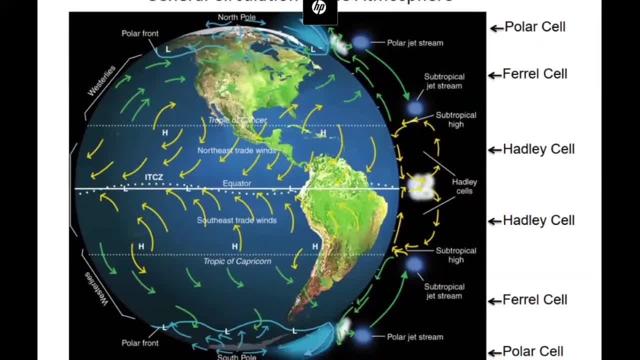 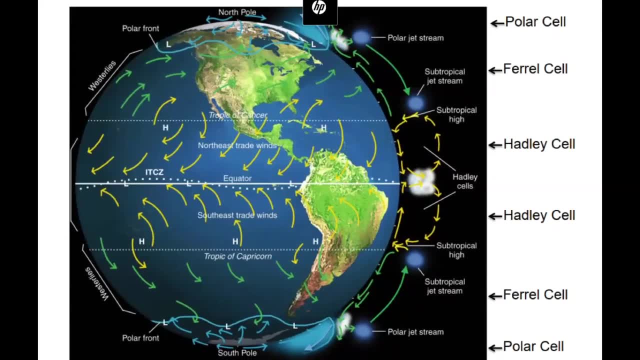 So people actually give names for each of these. For example, for the cell that's at the lower latitude, right near the equator, we call it Hadley's cell. So you can see that in the Hadley's cell the air is going. 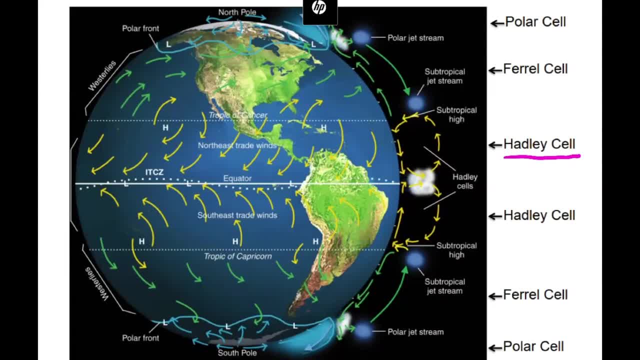 moving from north to the south and then rise up at the equator and then goes back at higher altitude and then settle down. okay, So the air is going to warm up mainly because the equator is the hottest, and so the air is going to go up in this way. 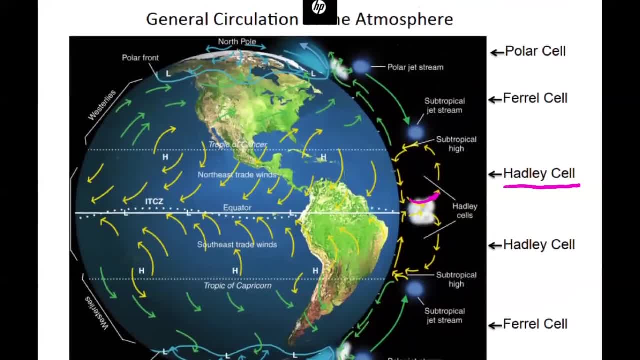 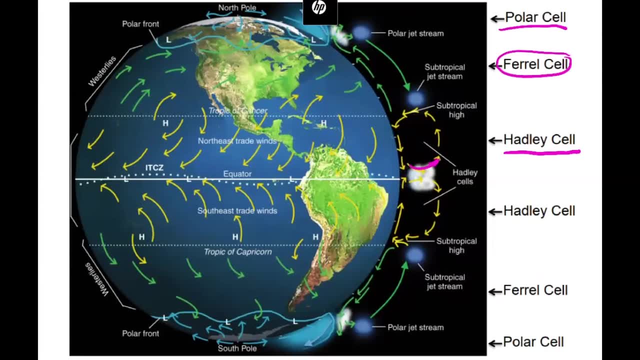 And in the polar region, which is a higher latitude region, we have this polar cell. And then we mentioned that the cell that's in the middle is because of the. it's basically it's generated due to these two different cells, due to the polar cell and the. 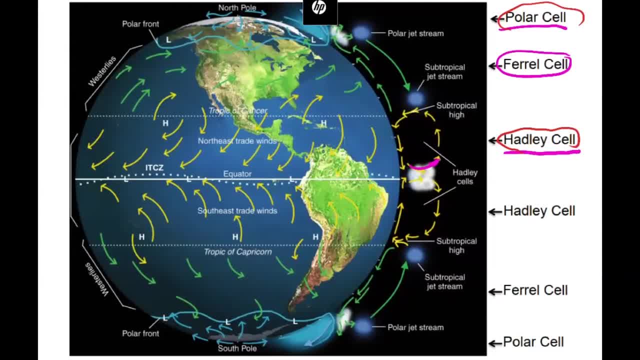 Hadley's cell. So basically, it's enforcing the air to recirculate in this way, right? So the air is going to go from south to the north, Near the surface, and then it's going to reverse at a higher altitude, at a higher height. okay, 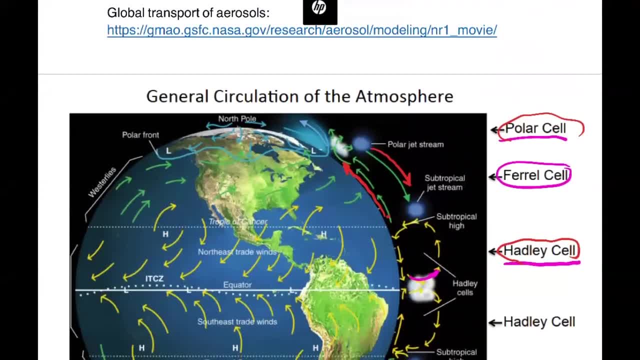 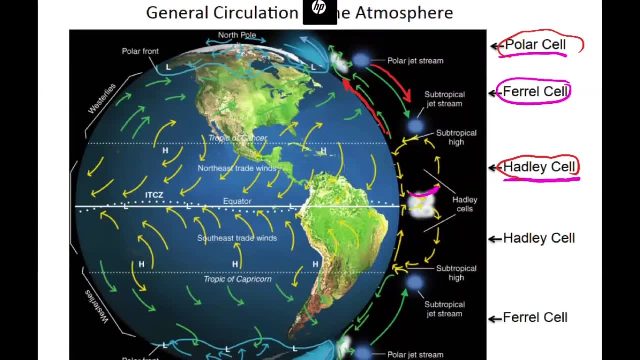 So, basically, due to the temperature difference, this is due to the solar radiation that we're going to have different air recirculations And this determines the wind direction from north to south or from south to north right, For example, in the polar region. 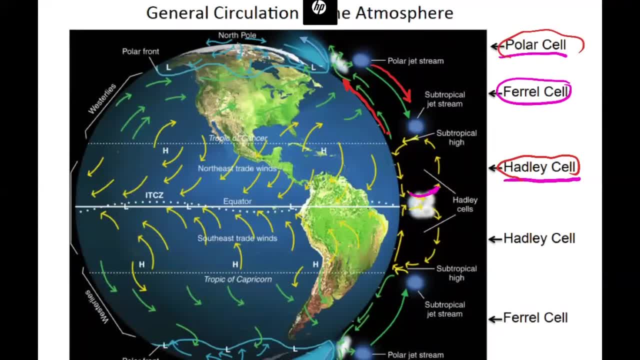 we're talking about the wind direction at the surface where people live, right. So the wind direction is going to be south to north And then in the mid-latitude. if you talk about the wind direction at the surface right, Then that's going to be south to north, right Having. 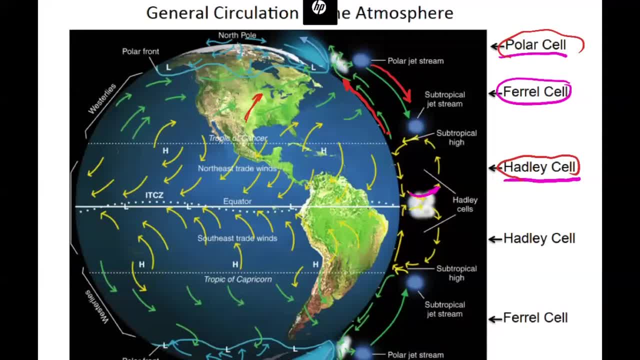 this direction. And then, if we're talking about the equator region, that's going to be south, that's going to be north to south, again going to be this direction, okay. So then we may wonder: this temperature difference, this air recirculation, only determines the wind direction. 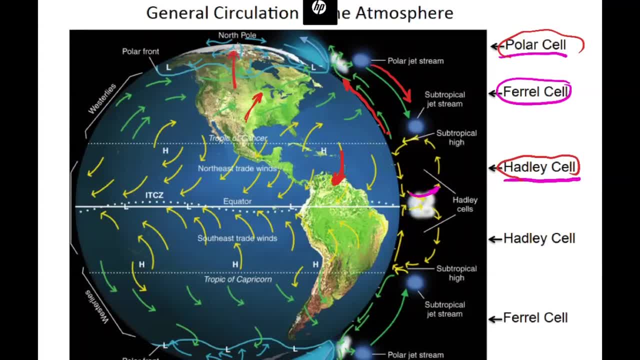 in the north to south direction right. So it's either north or south. So what about the wind direction? from east to west or west to east? We mentioned that near the equator region the wind direction is from east to west, right. So why do we have this direction of the wind? 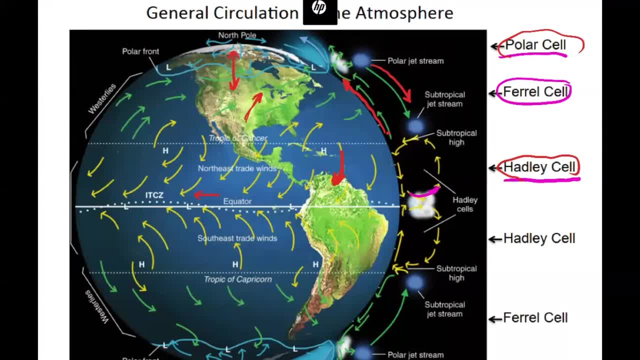 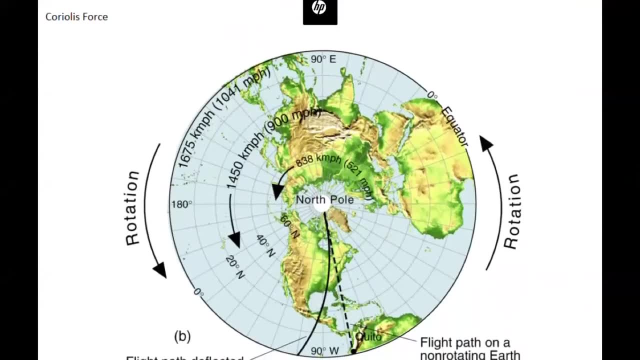 And the wind direction that's along the rotation direction or the rotating direction of the earth, is mainly caused by the Coriolis force. I think you probably have heard of this force in your physics classes. okay, So the easier way to introduce this Coriolis force: 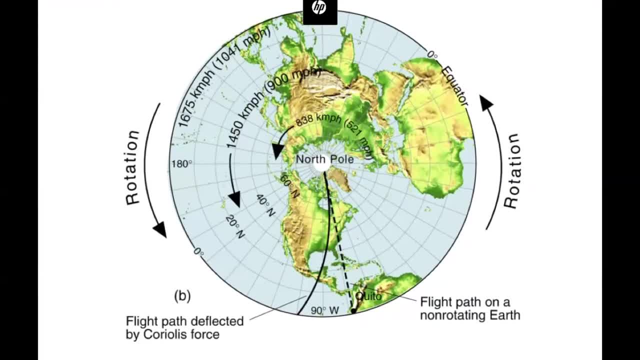 is to just, let's say, if we just look at the earth from the North Pole, right, So this is showing all the different continents, right, You have the North America, Asia and part of the Africa. okay, So an easier way to understand the Coriolis force is: let's imagine that you're standing here. 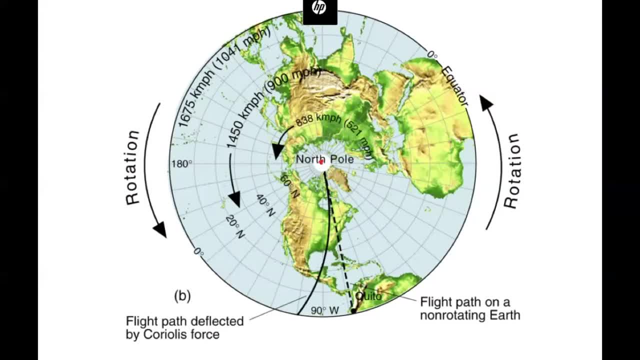 on the tip of ice- okay, on the North Pole. and then you decide to throw a dart- okay, So, since you are not at the North Pole, so no matter which direction you are throwing this dart, it's always going south- right, Let's say that we're throwing this dart. 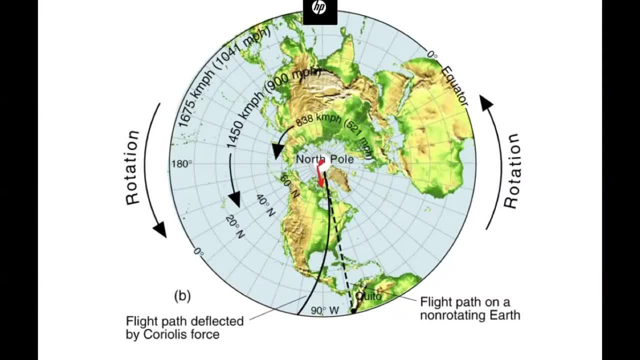 so hard that it's going to float in the air for some time. okay, So because of the rotation of the earth, which is from west to east. so because of the rotation of the earth. so when you throw the dart out, you don't have any. 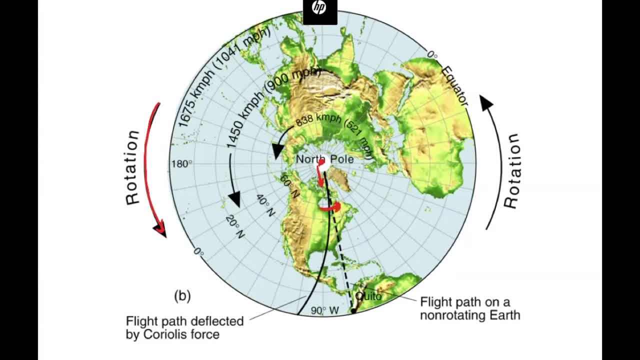 force that's being applied onto this direction, right, You only have the force being applied from north to south. So, because the earth is rotating in this direction, so the earth will move faster compared to the dart that you throw out, right? So then you can imagine as the dart is flying on the air: right, because of the earth. 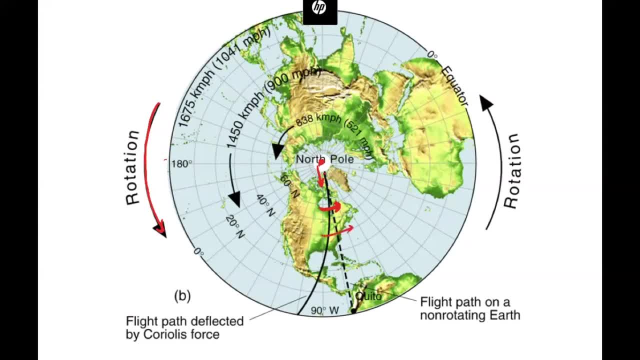 it's moving much faster compared to the dart in the west to east direction. So the dart is going to gradually deviate from its original trajectory and then it's going to go this way right. So it's mainly because our earth is having its 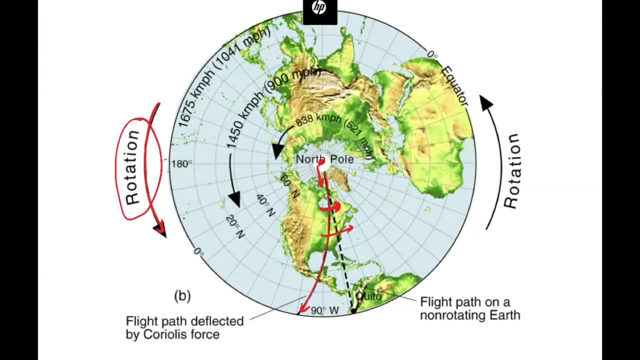 rotation from the west to east right. And since we, when we throw all the dart, we don't have any direction in terms of the west to east directions. So gradually, we're going to deviate from our original trajectory. So which means that if you're 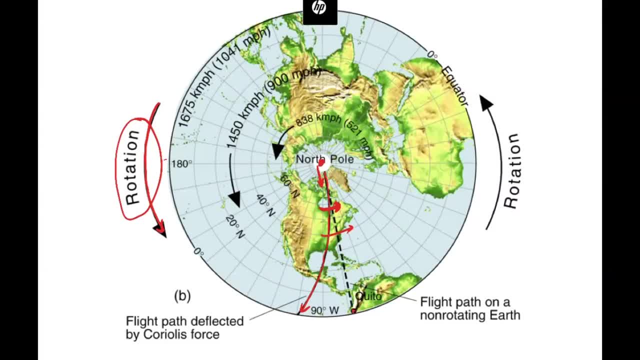 trying to throw this dart, aiming at Quito, right, This is a city in Chile, right? And then, because of the earth rotation, the direction is going to deviate or it's going to bias towards the right of its original direction. okay, So this is because of the Earth's rotation. 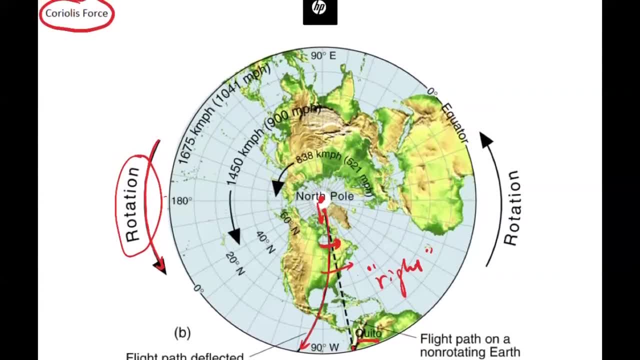 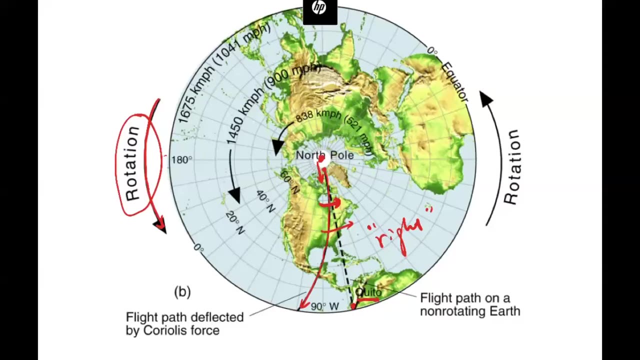 and if you want to calculate how much it deviates from its original trajectory, you will have to use the detailed form of the Coriolis force. okay, So the same thing will happen if you're trying to throw this dart from Quito towards North Pole. okay, So now, if you think, 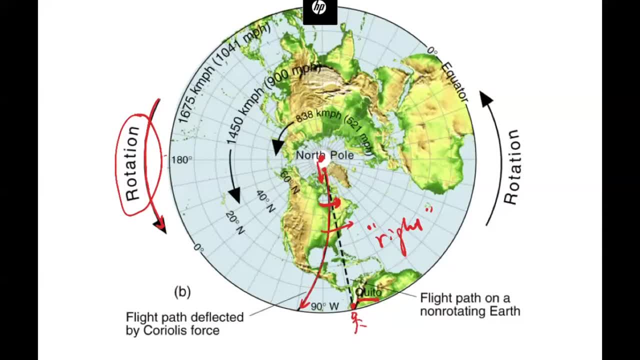 about the scenario where you're standing here and then trying to throw a dart aiming at the North Pole. okay, So just think about immediately when you throw this dart out, then you're basically having a direction that's towards the North and also you have a velocity that's moving. 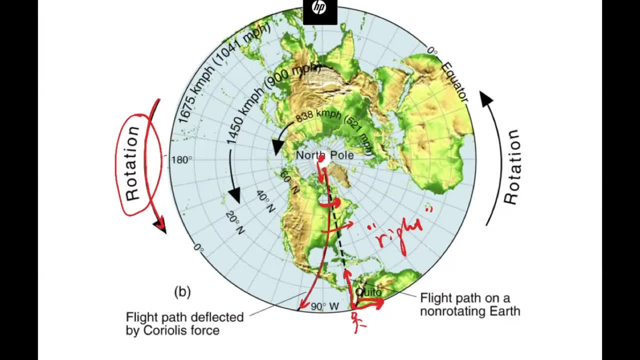 out together with the earth right, and we know that the the speed at the equator is going to be the fastest right, and then what that means is the dart is going to have an extra velocity. that's basically falling from the west to east direction and as the dart goes towards the north pole, 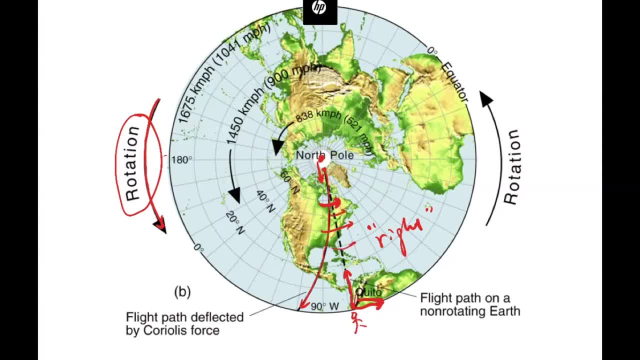 since the earth at a higher latitude, it's moving, a moving with a slower speed. so what that means is the dart is going to gradually deviate from its original trajectory and then go this way. so this is mainly because the dart that you throw out at the equator has a faster speed. 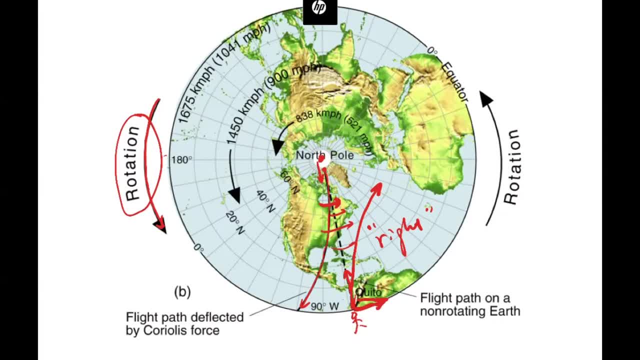 from the west to east. okay, and the result of this movement is also: the dart is going to deviate or bias towards the right, and this happens for all of the movement on the northern hemisphere. okay, so no matter whether you throw a dart, let's say following the following: this direction: right, west to west, to east. 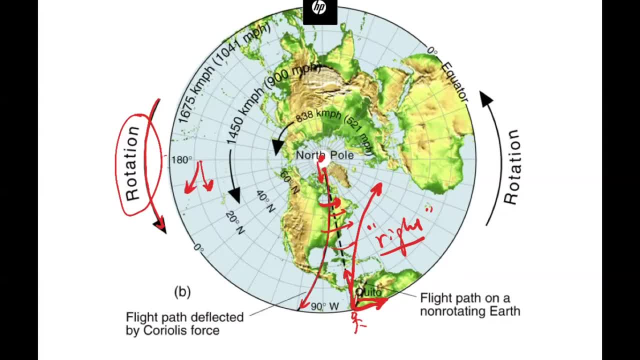 direction. the dart is going to deviate towards right of the original direction and then if you throw a dart in this direction, then the actual trajectory will go this way. okay, so this happens to all of the movement on the northern hand hand hemisphere. in terms of the southern hemisphere, the things will be reversed. what happens is: 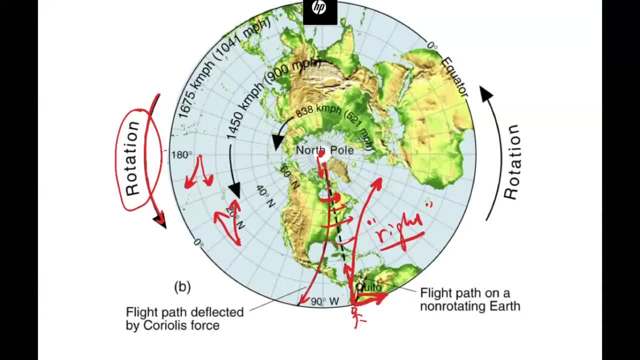 basically, if we throw a dart from the south pole towards the equator, then this dart is going to bias to the left. okay. so if i write it out in the northern hemisphere it's going to bias to the right. in the southern hemisphere it's going to bias to the left. 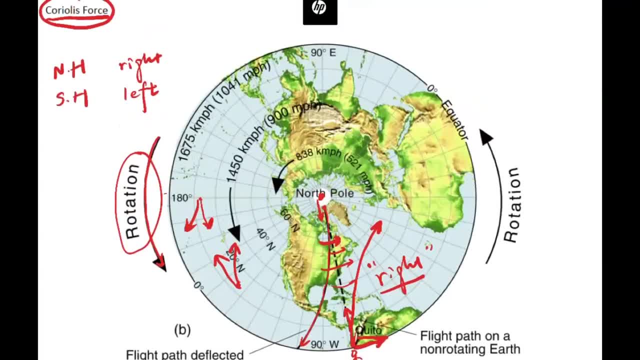 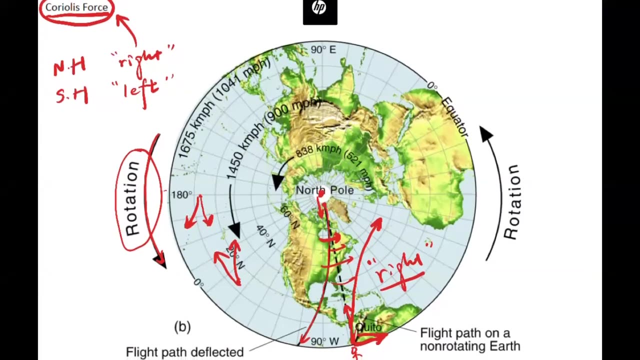 okay. and this deviation from its original trajectory is caused by the coriolis force. and if you feel that it's quite difficult to memorize which direction it is, i think a simple way to memorize it is: you can think that because we're living on the northern hemisphere, so we're 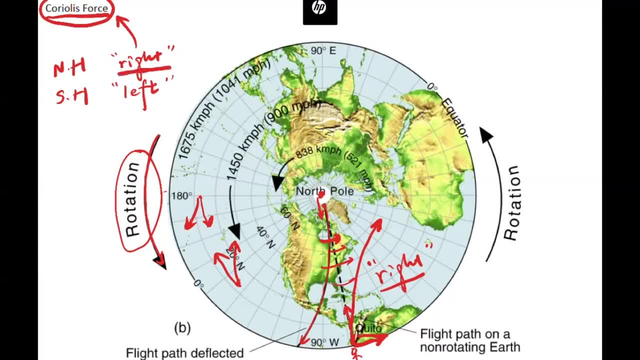 always right. okay, so we're always biased to them, to the right. so it doesn't mean that we're always. It doesn't mean that people leaving on the southern hemisphere they're wrong, It's just their bias to the left. Okay, So this is an easier way to understand the direction of the Coriolis force. 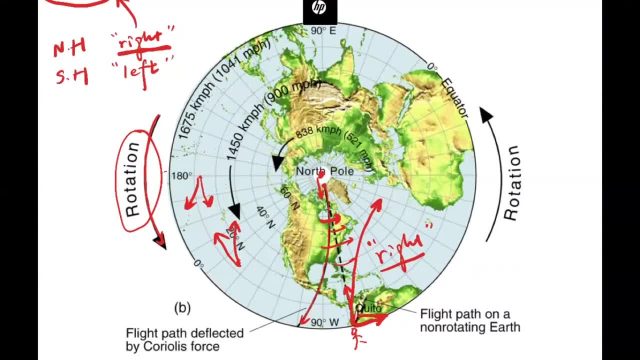 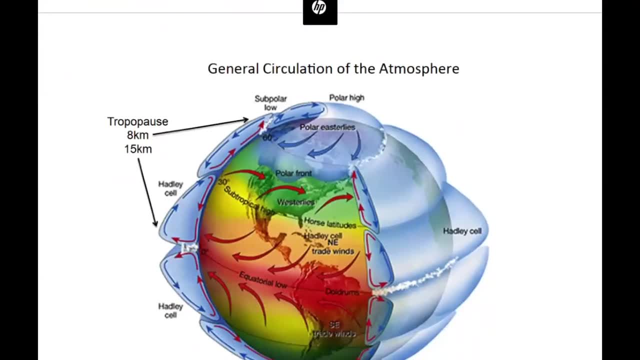 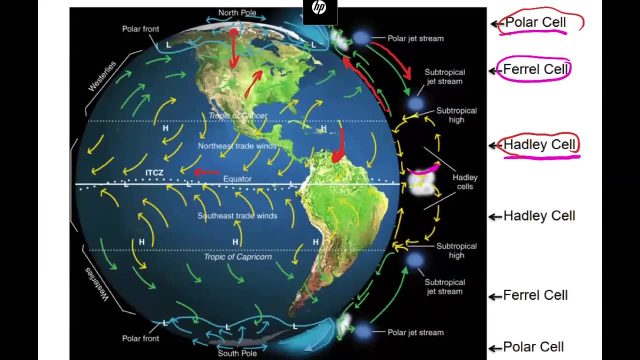 And now you can think or think of, think about the wind direction globally and things are going to explain themselves. Okay, so let's see if we go back to the previous picture here. So we mentioned that the wind at the lower latitude Right Was close to the equator region. The wind is going to flow from south to from north to south right, mainly because the equator is has a higher temperature. 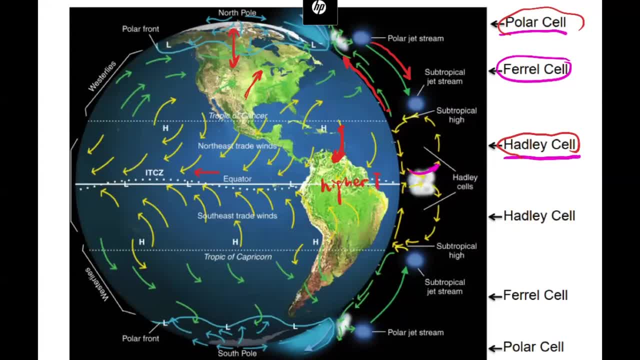 Right, So the air is going to rise up, right, it's going to create a lower pressure region at the surface, And that's why the wind is going to floating, going to flow from north to south to fill in this low pressure zone, right, so, while it's flowing from, 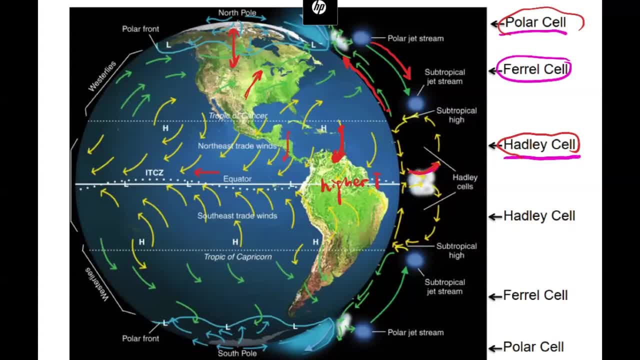 north to south. due to the Coriolis force, it's going to bias towards the right direction, going to go this way, right, and that's why, in terms of the general wind pattern near the equator, you're going to have the wind direction from east to the west. 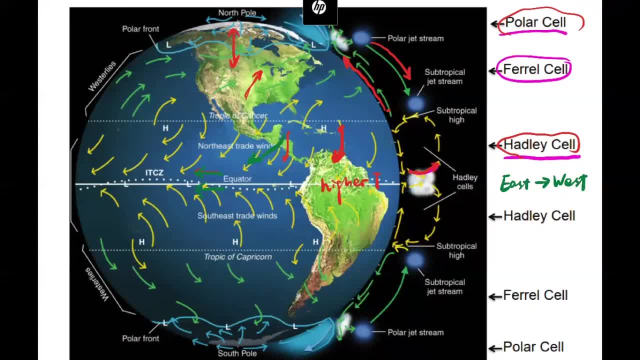 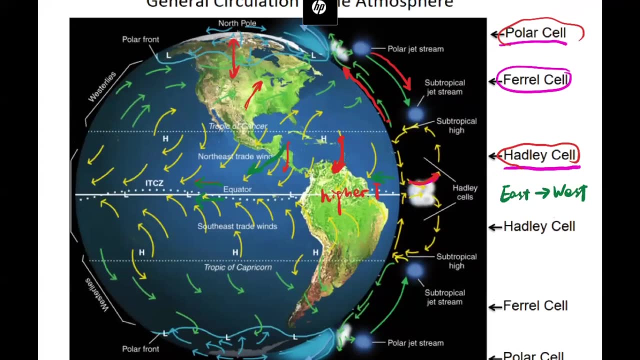 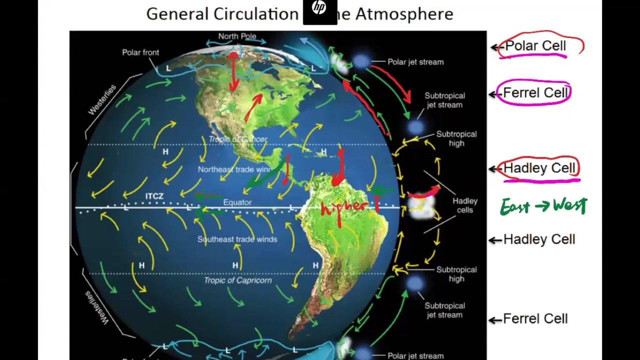 so that's why, also, the dust from the Saharan desert are going to transport all of those, all of those dust particles towards this direction, right, and the same thing happens for the mid latitude where the United States is located. okay, so we mentioned that in the mid latitude um the air, because of the Farel cell, 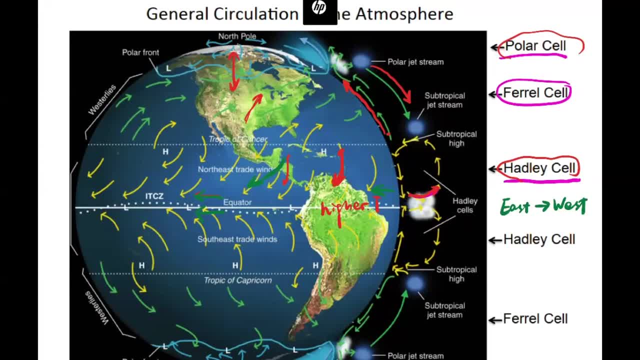 right. so the air is going to move from south to north. at a surface it's going to go this way and because the air or the movement is bias to the right, so we're going to have the general wind pattern that's going this way. this is at the surface right and now, if i ask you a 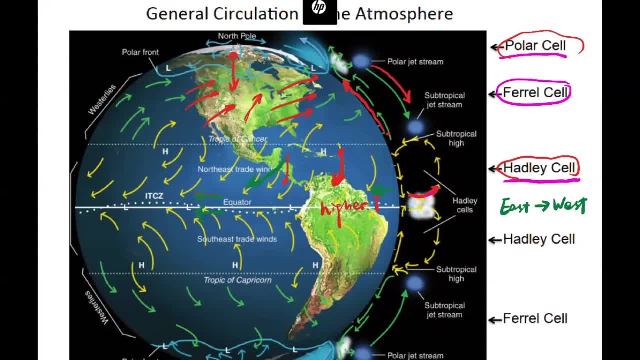 question: if we decide to build several nuclear power plant- okay, we want to just build several nuclear power plant in the united states- where should we put them? should we put them at the west coast or should we put them at the east coast? we should put them at the east coast, right? so we want to do that. 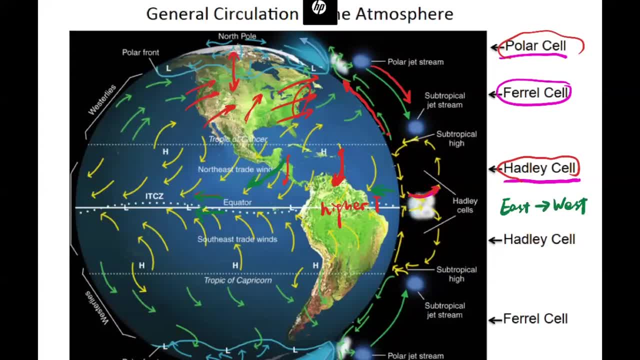 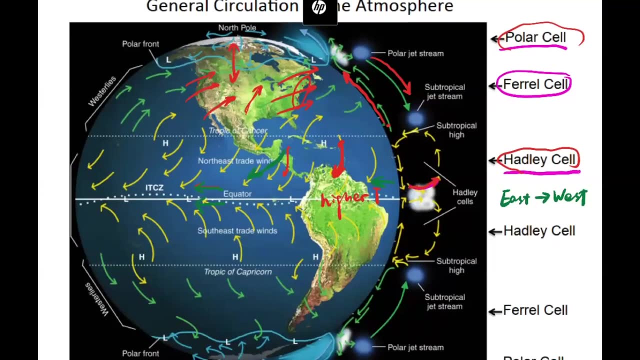 mainly because, even if there is something bad happens, let's say tsunami happen, if you think back on the accident or the the disaster in japan 10 years ago. right, even if those things happens, even if we release the radioactive materials, so the air is still going to transport all of. 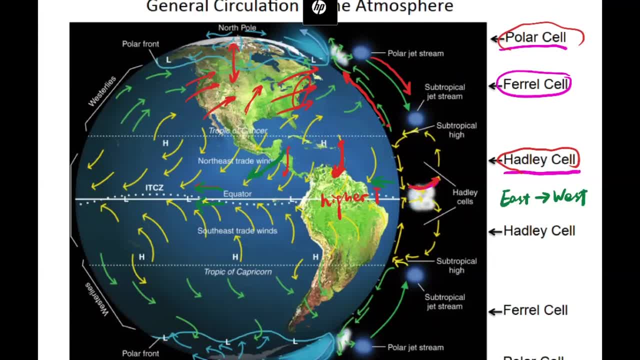 those hazardous material towards the east right. it's not going to float over the united states, it's not going to harm the people living here directly. okay, so that's why, um, the meteorology plays a lot of important roles in the air pollution control. so, mainly because, if you 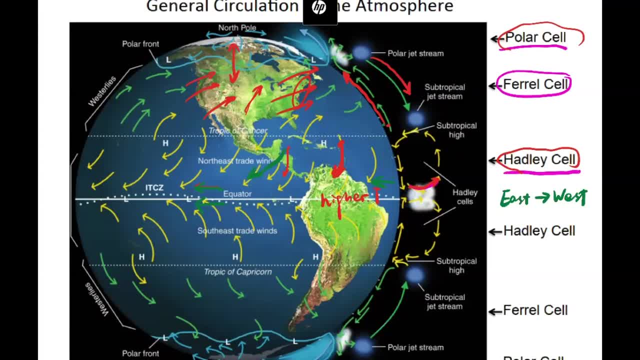 think about the general wind pattern at the east coast, right? so it's most of the most of the time the wind is going to blow from west to east and this is going to decide that we consider the transport of the air pollutant. it's just going to transport all of these pollutants over the ocean. 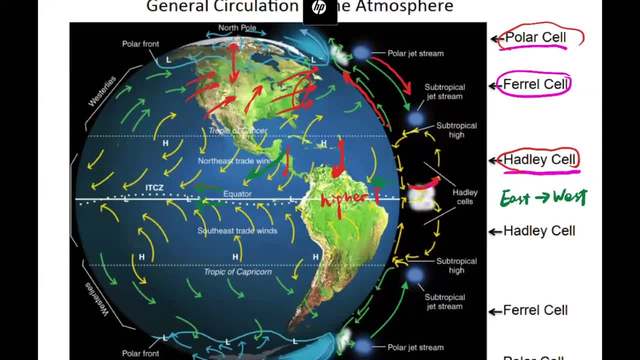 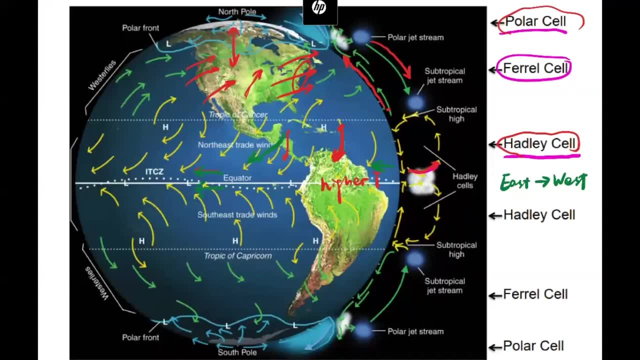 where no, uh no other people live on there, right, so we can be less concerned about the air pollution problem, right? so basically, it's because of the temperature difference on the earth and also because of the coriolis force, we're going to have this general wind pattern, or the global wind pattern, in. 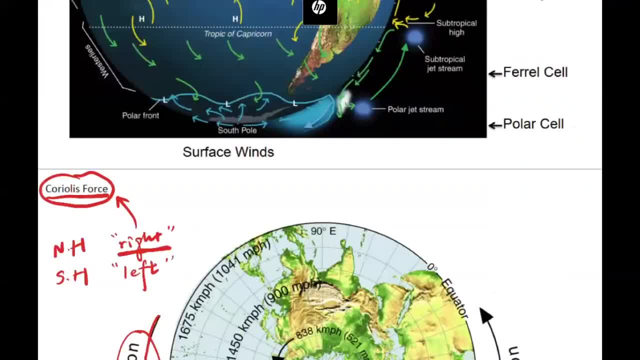 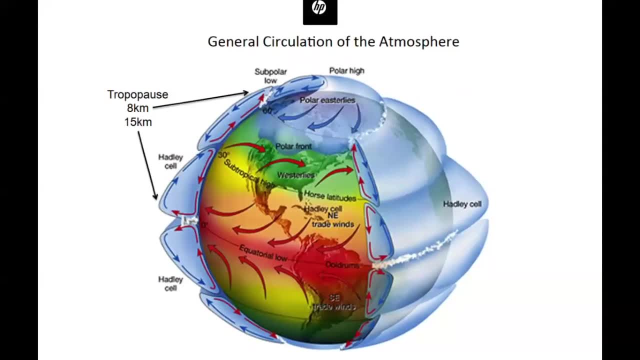 different cells of our earth. okay, so it also has some applications, and here i'll just reiterate what are. how are these cells look like? okay, so we have the hydrogen and the hydrogen and the hydrogen. we have the hadley cell, which is a cell near the equator's right, and then we have the farrell cell. 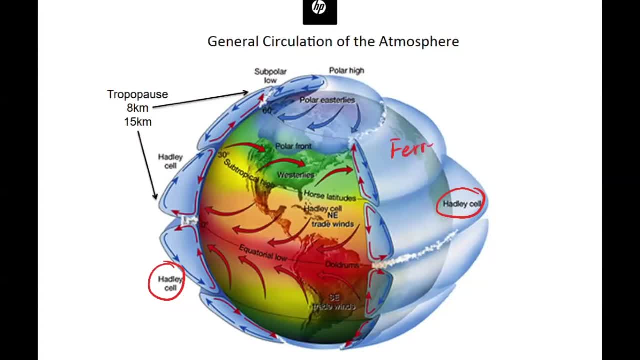 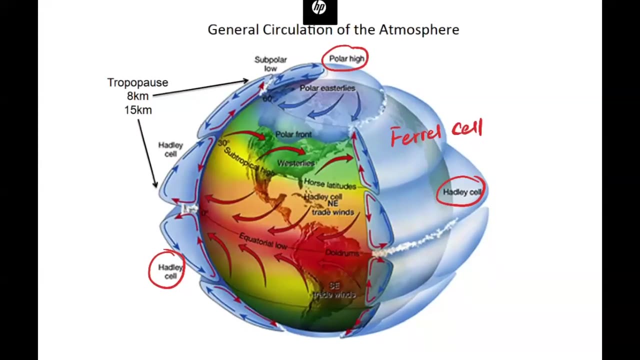 i don't think it mentioned here. okay, it's basically the cell at the mid latitude and we have the polar cell at the higher latitude, and if you further look at the thickness of these cells, you can see that the cell are most thick. the cell is the thickest at the equator region. okay, so the air can rise up and then can reach to an. 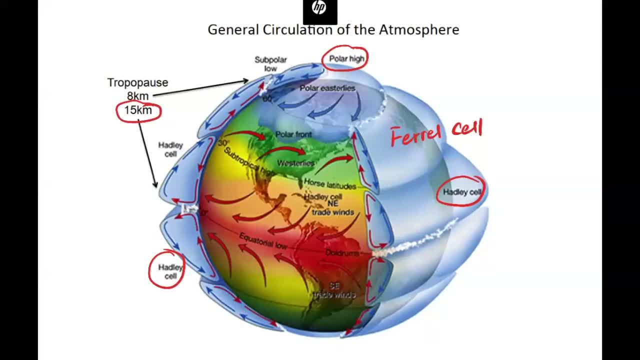 altitude of around 15 kilometers, and this is mainly because the temperature here is so high, so the air has a lot of momentum, has a lot of heat to rise up to the higher altitude. if you compare the thickness of the cell at the polar region, so basically that's going to be much thinner, right. 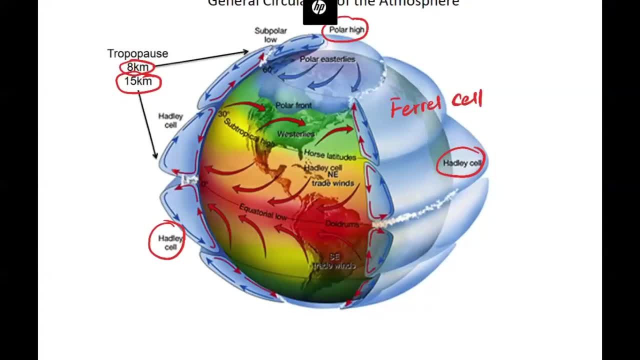 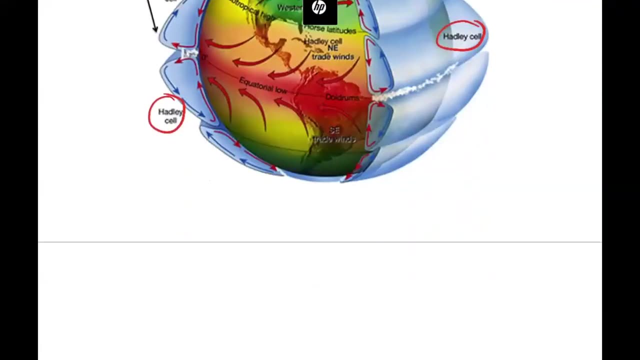 and then it's around eight kilometers high. okay, so, mainly because the air here is very cold, so even if it rise up, it's going not going to rise up for a large altitude here. okay, so, um, this is how all of these cells look like, and it's going to have a lot of applications. 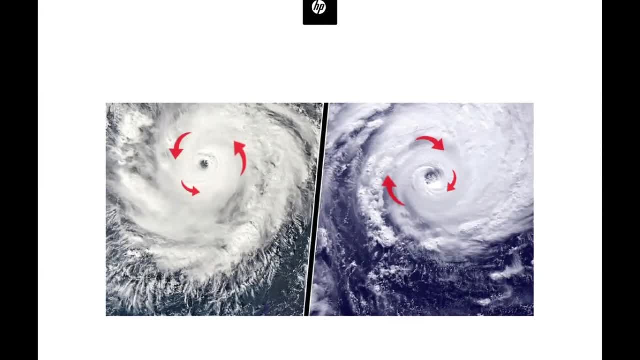 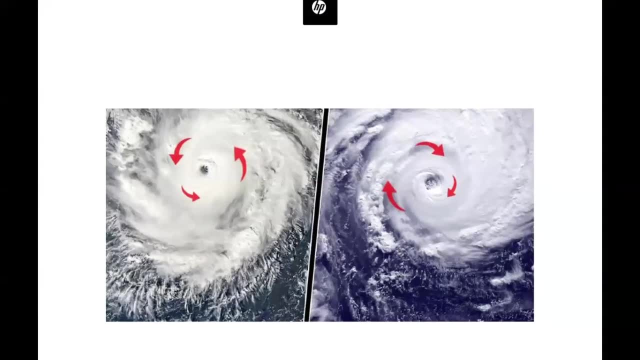 as i mentioned, and one application is the direction of the hurricanes. okay, so here i'm showing two hurricanes. um, i can tell you that one is coming from the northern hemisphere and one is coming from the southern hemisphere. so if i give you a quiz and can you tell me? 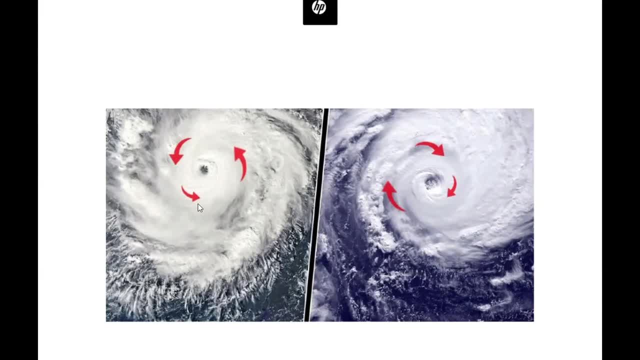 which hemisphere is the first hurricane located? is it in the northern hemisphere or is it in the southern hemisphere? and just take a guess. Okay, All of you have responded. It is the northern hemisphere. Okay, And I think most of you have got the correct answer. So the direction or the rotation of the hurricane. 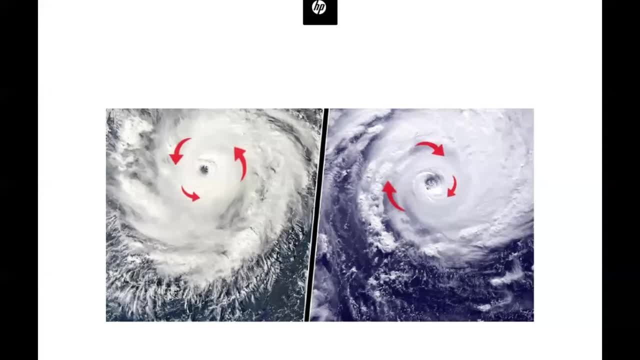 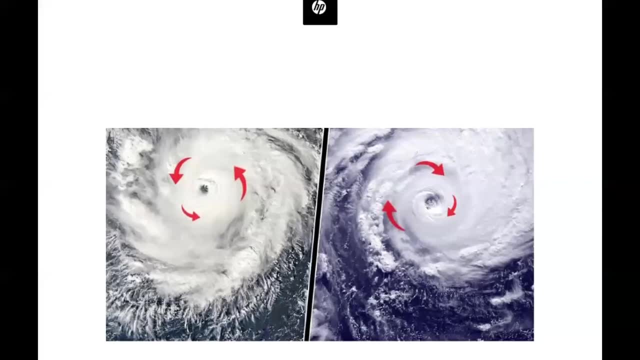 system is also dependent on the Coriolis force And the reason for its formation is also because of the pressure difference, right? So whenever we mention about the hurricane, if you just look from this direction- let's say look from the horizontal direction- So what happens? 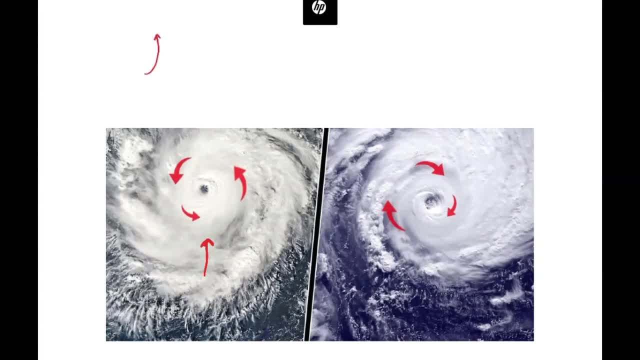 is, we have a low pressure center that's trying to move the air towards the higher altitude. Let's say this is the ocean. So basically we have a very low pressure center for this air movement. So a lot of air are going to move to the higher altitude And then because of the higher altitude, because 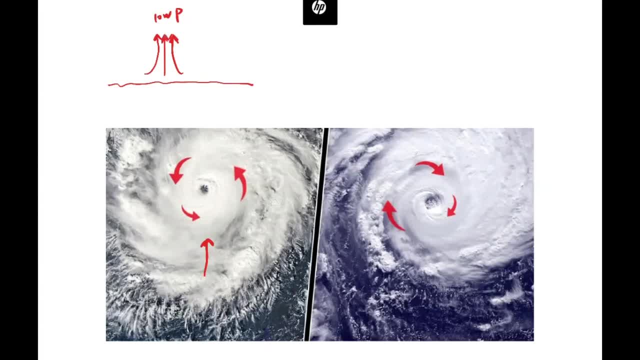 of the upward movement. so all of these moist air, moist air over the sea water, are going to be transported upwards. And then we mentioned that at this higher height here it's going high. So the temperature is lower, right, So the temperature is lower, and then they're. 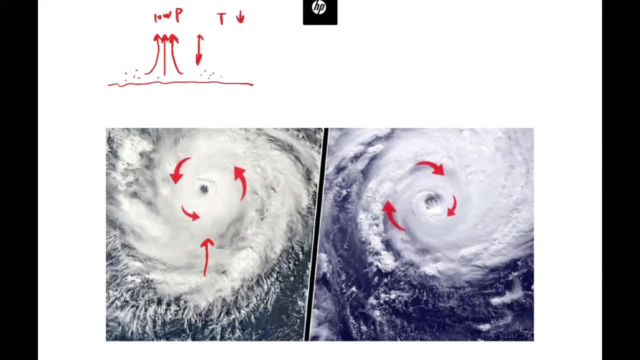 going to condense a lot of water. that is going to form an intense cloud and also intense rainfall, right. So this is what happens during a hurricane. So what this means is that, when the air moves upso, this low pressure zone is going to get transported towards the surface of the ocean right And 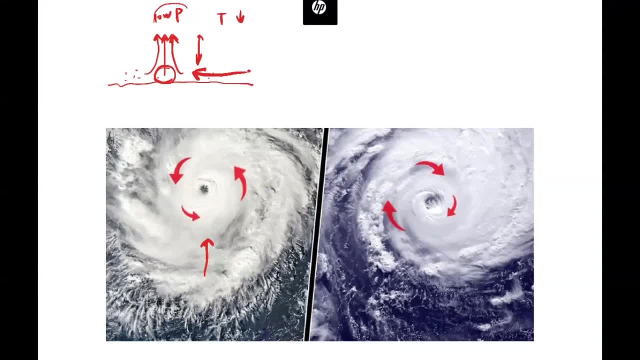 � . OK. And because of low pressure zone, a lot of air are going to move from all of the directions towards the center, okay? From any direction, mainly because we have a very low pressure at the center here. So now we can start to look from the angle that's up of the hurricane. 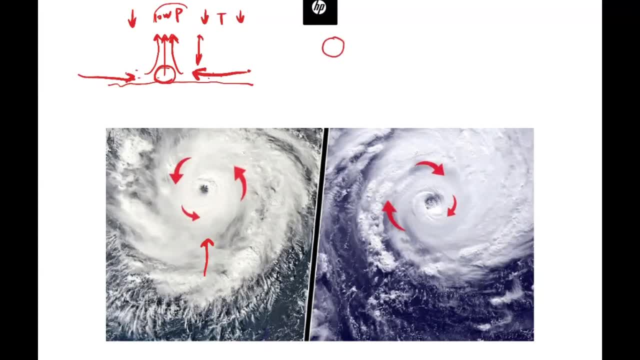 So what happens is we have a very low pressure center right And the wind is going to go this way right, And this is the targeted direction. okay, This is our, if you think back on the problem for throwing a dart. 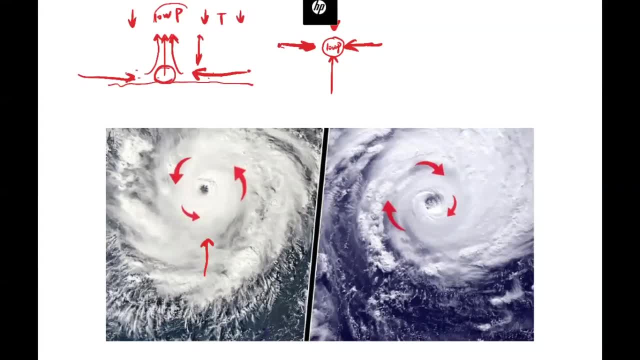 So this is the direction of the dart that we aim at: right. And now, if we're at the northern hemisphere, one thing we mentioned is that all of these wind are going to bias towards the right. okay, If it's biased to the right. 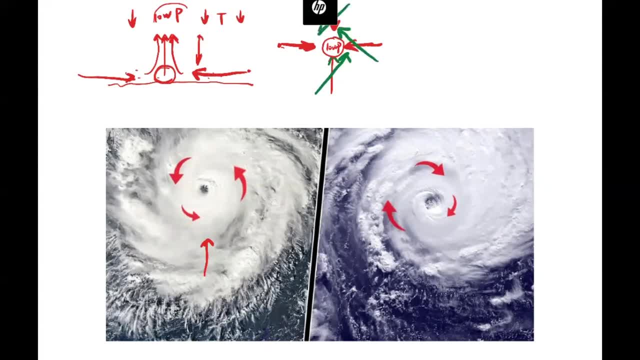 It's going to go this way, right And now, because the air are going to compress each other, right, They're not going to go directly or this in this straight direction, They're going to go this direction, okay. And now we can tell that this is counterclockwise, okay. 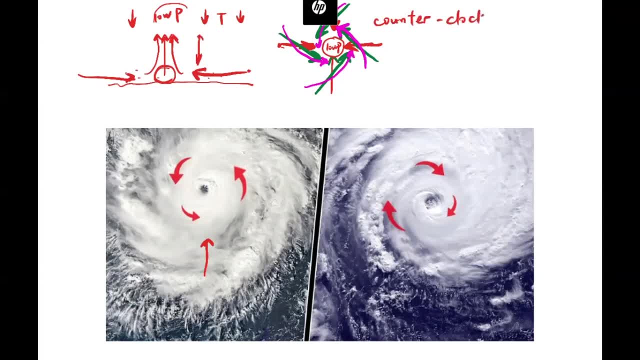 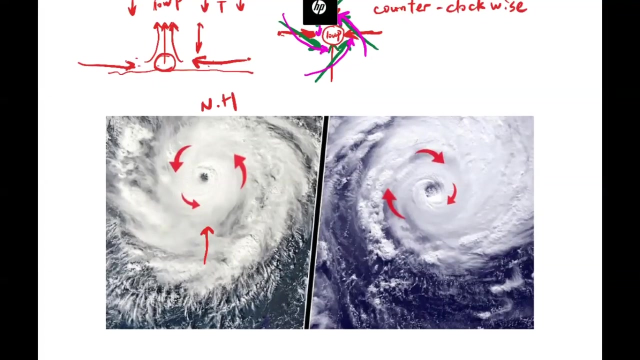 Okay, And if you look at these two hurricane systems, so the first one is counterclockwise, which means that we're at the. I mean, basically this hurricane system is at the northern hemisphere And then, because of that, this hurricane that has the clockwise direction is at the southern. 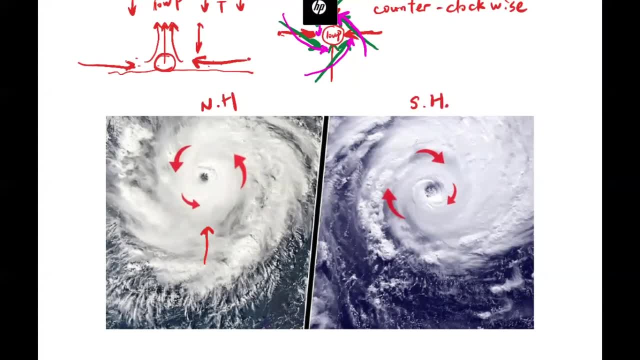 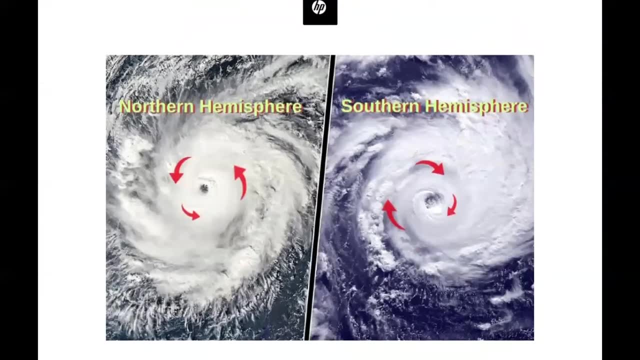 hemisphere. okay, So this is how we can tell whether a hurricane system is at the north or at the south, And I want to say that this is the correct answer. okay, So I want to say that I'm not making this up, okay. 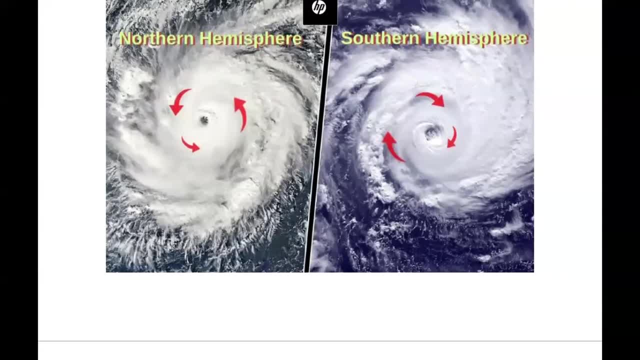 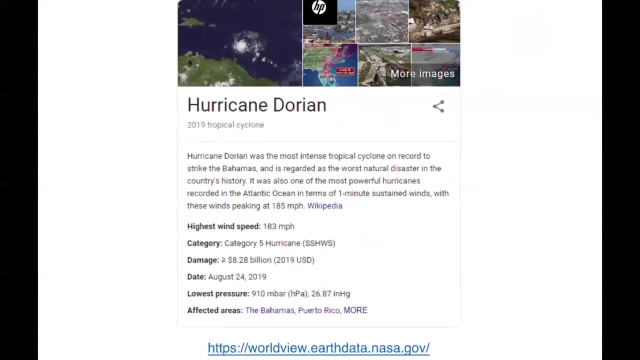 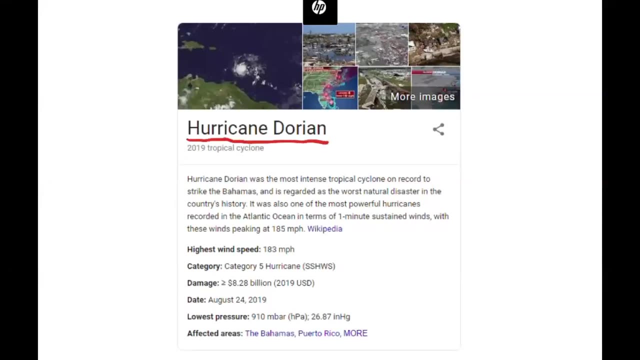 I didn't just search for two hurricane systems and then tell you which, where it's located. So basically there are some examples we can look at. So here I'm showing the hurricane system. Okay, This is the hurricane Dorian, so this is basically the strongest or the most intense tropical. 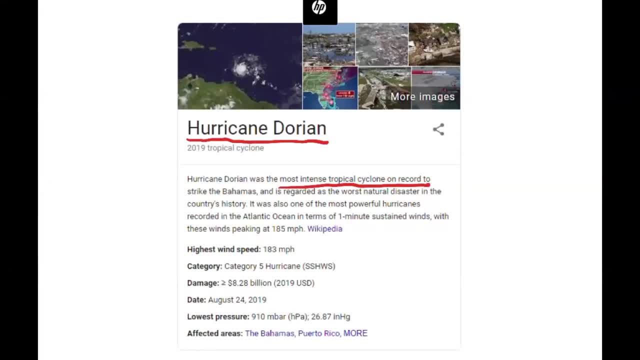 cyclone on record. okay, And this happened last year. I think this year there weren't many strong hurricane system, but last year there are a lot of these hurricane systems that's harassing the tropical region and also the southeast of the US. okay. 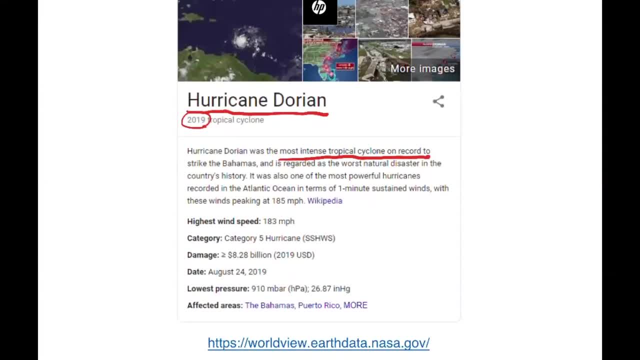 So, basically, we can try to track this hurricane system. So this is the hurricane system based on the, based on the NASA satellites, and here I have a link which is showing the satellite images that's collected on all of these, from all of these platforms. 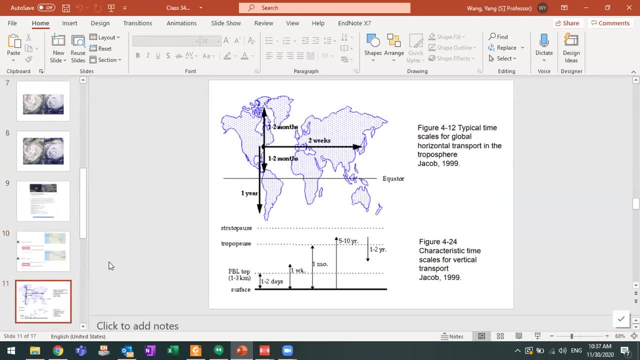 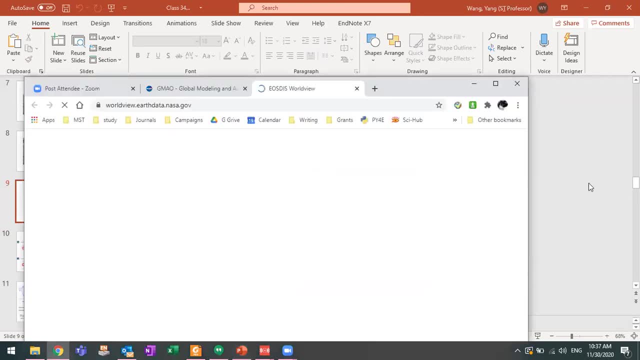 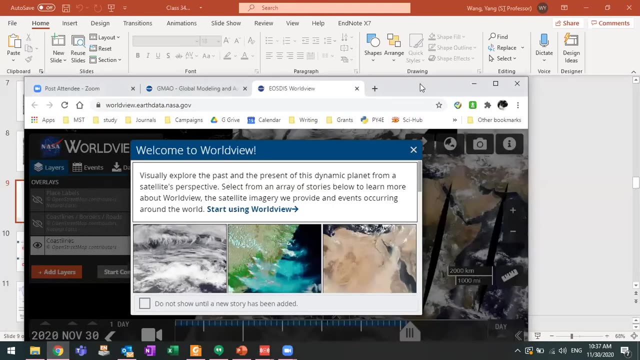 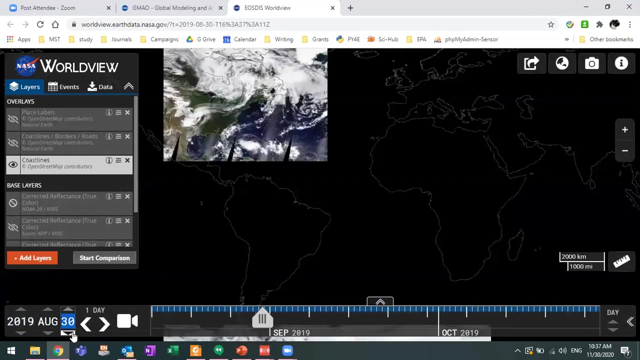 So let's say, if we just try to go to this link here, So if you pay attention to the date of this hurricane, this is August 24th 2020.. Okay, So, if you just jump back to that date, okay, so this is how we can track the hurricane. 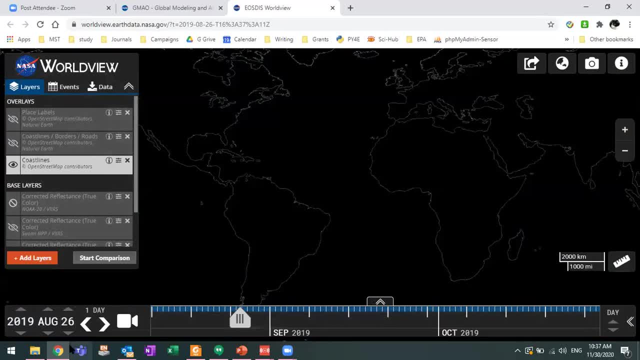 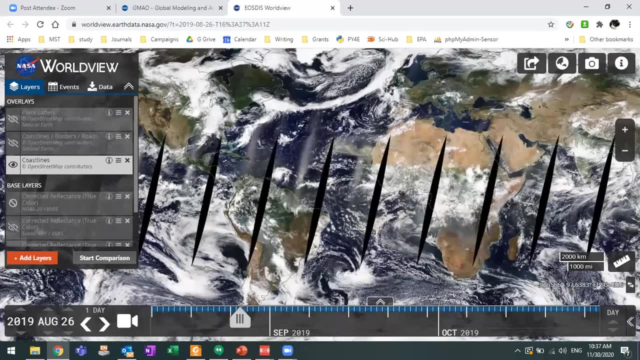 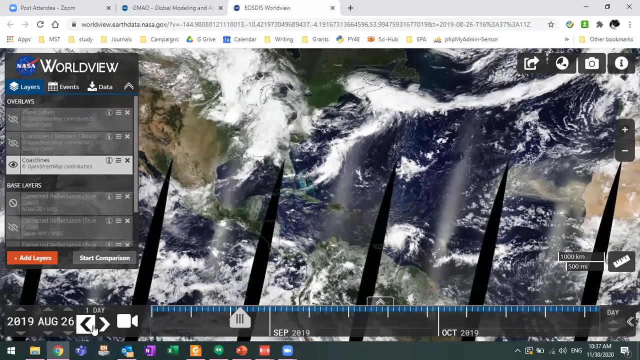 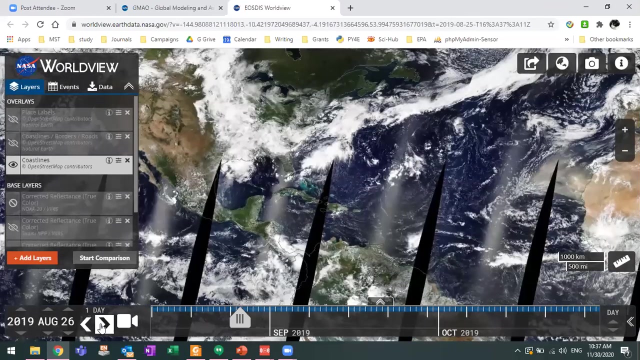 Dorian, And I think, let's see, this is August 24th, right? So if we zoom in to this area, So I think this is the start of this hurricane, okay, So it started from here, right 24th, and then started to grow, right. 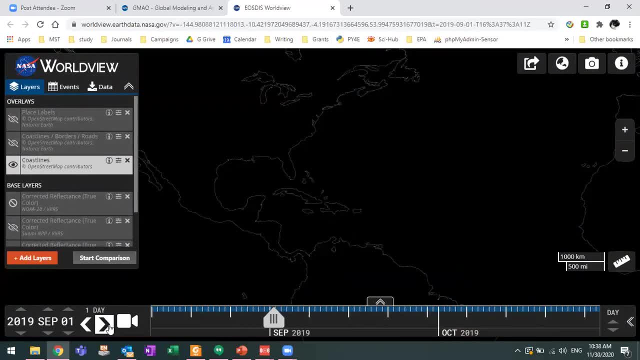 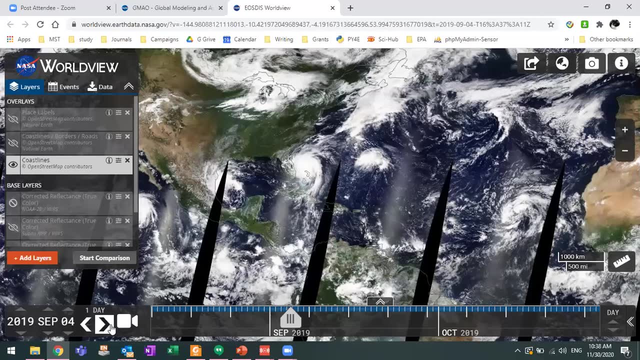 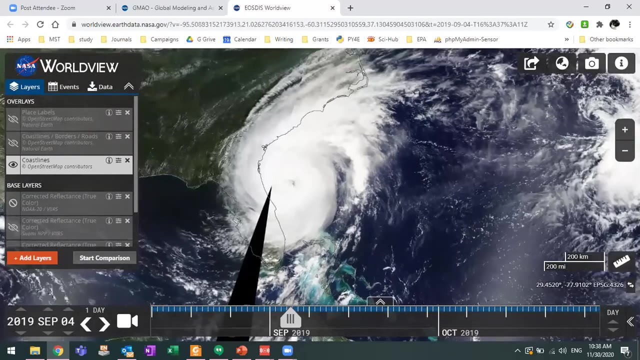 You can see how it grows here. It grows larger, larger and larger, And now it hits Florida. All right, So now, if you pay attention to this, this is August 24th 2020.. So now, if you pay attention to the direction of this hurricane, you can see this is counterclockwise. 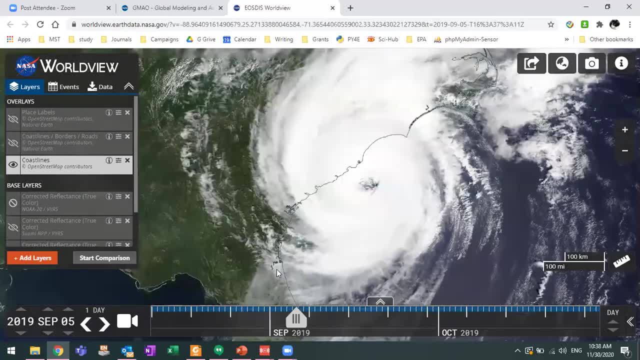 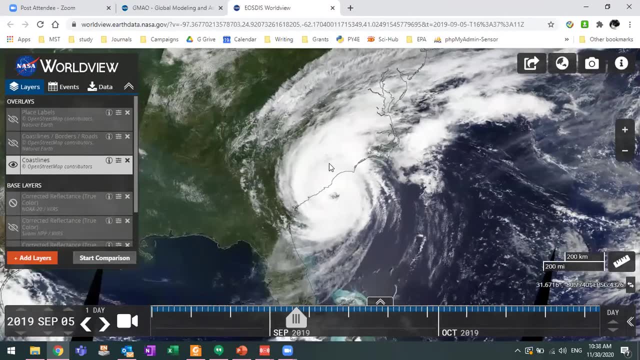 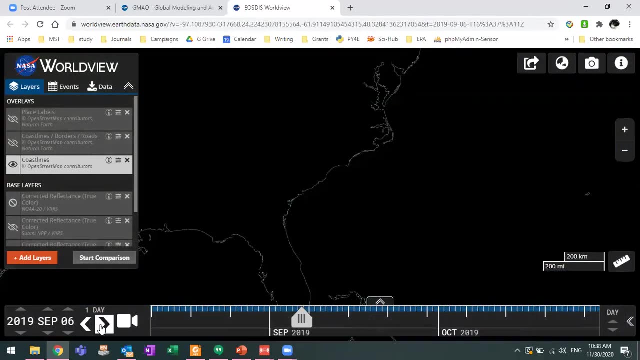 Okay, Right, This is mainly because this is the northern hemisphere And you can also see, this hurricane is in a very, very large scale. right, It has a size of almost that of the Florida, Okay, And the wind is also very thick. 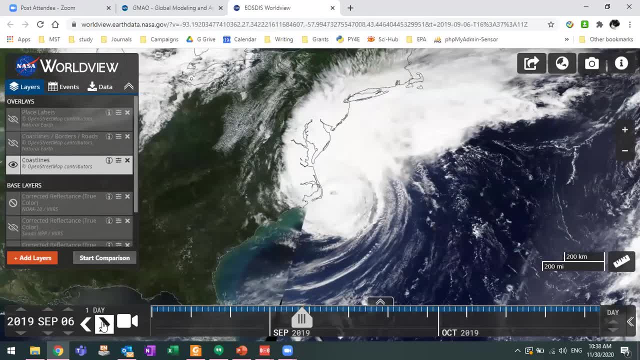 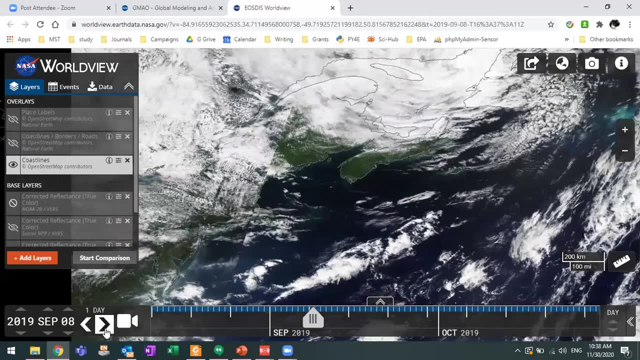 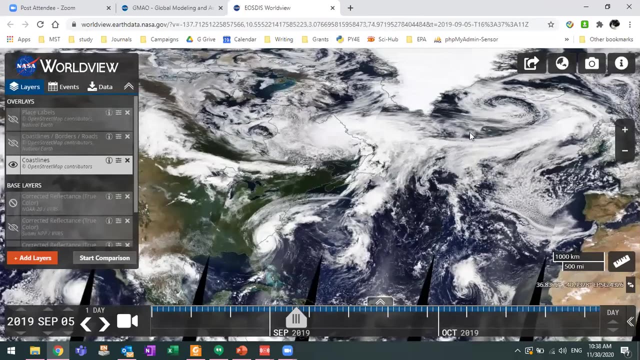 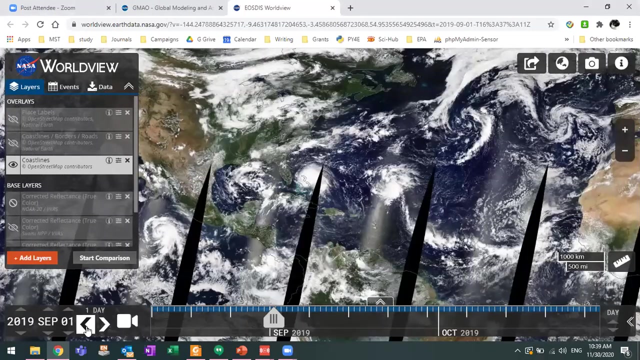 It's causing a lot of damage To the people living near the coast. Okay, Further it moves to the New York area Right. And also, if you try to track the movement of this hurricane system, you see it's being generated from the equator region. 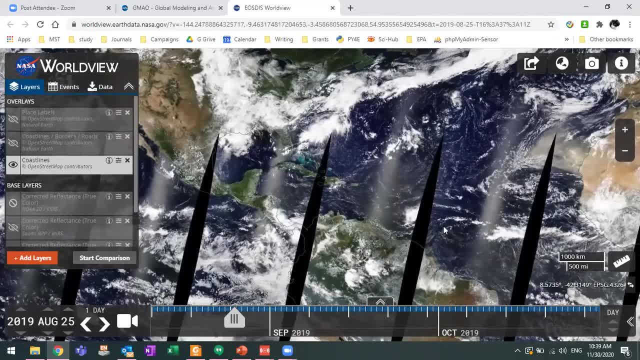 Right, So we see that the equator is here. So when it's being transported, when it moves itself first, it moves from east to the west. Okay, If you think back on the direction of the wind, that's happening at the equator. Right. We mentioned that the wind direction of the equator is from east to the west Right, So that's why it's moving in this way. And then, once it hits the mid latitude, where is the region of the United States Then switching its direction? 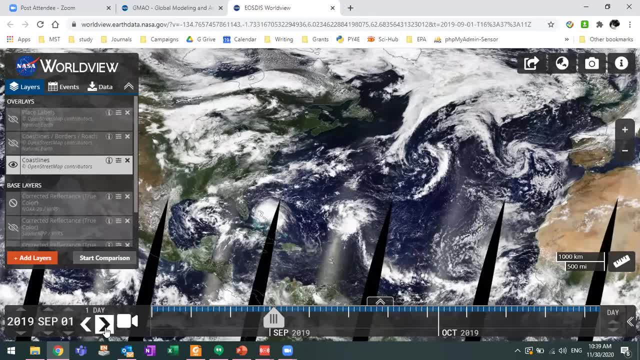 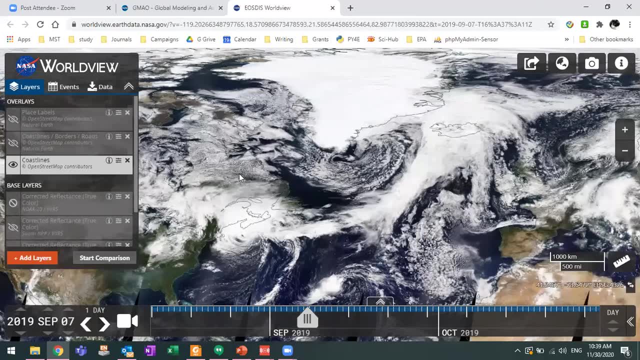 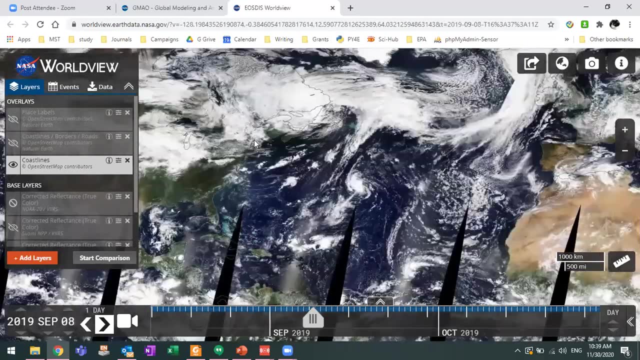 And then start to move from west to the east. So even the movement of this hurricane is following the, is following the Coriolis force Right. It's following the general wind pattern of the of the earth Right. You see, once this hits to the mid latitude, it starts to diverge the direction and then start to move from the west to the east. 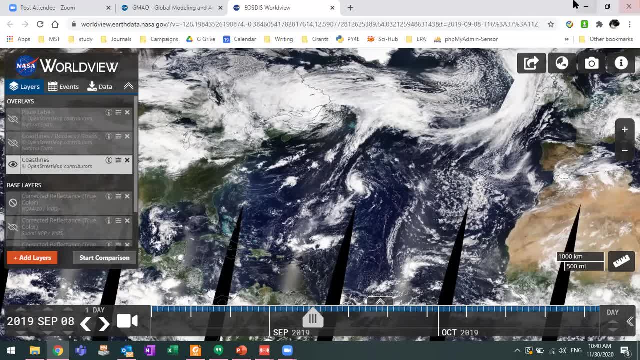 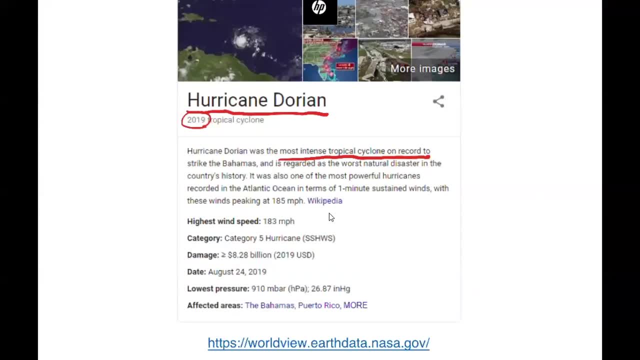 Okay, So it's not going to penetrate further Towards the center of the United States, Right? So this is very important information when people are trying to forecast the movement of the hurricane systems And we can use basically use a similar information to predict how the air pollutant moves, based on this global wind transport pattern. 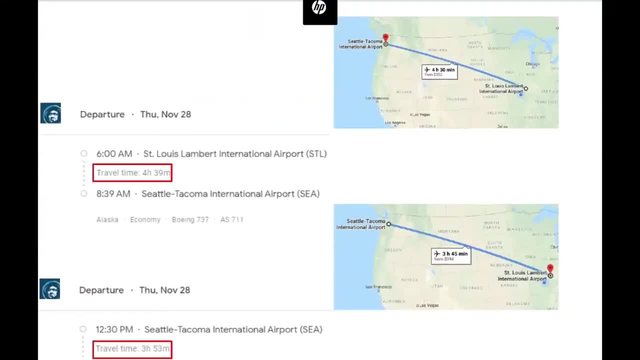 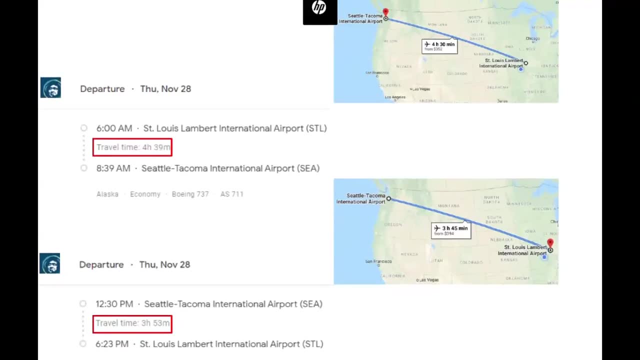 So there's another application of this Coriolis force. So I'm not sure if you have the experience of taking very long flights Generally in the United States. I refer to the flights that's flying either from either towards the west coast or the east coast. 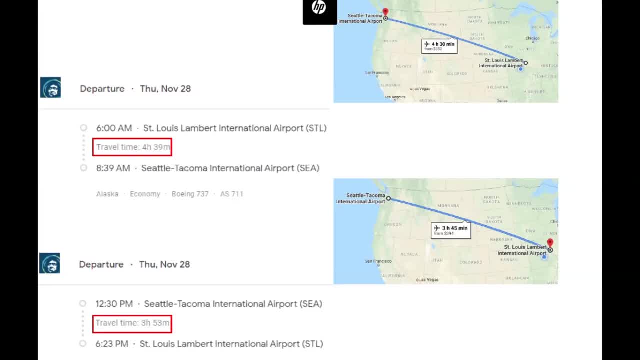 Okay So let's say, if we decide to drive to St Louis and take a flight to Seattle, Okay So normally, if you track them, just take a search on the Google flights. You can search for both ways. Normally what you can find is that if you try to fly from St Louis to Seattle, that normally take four and a half hours. 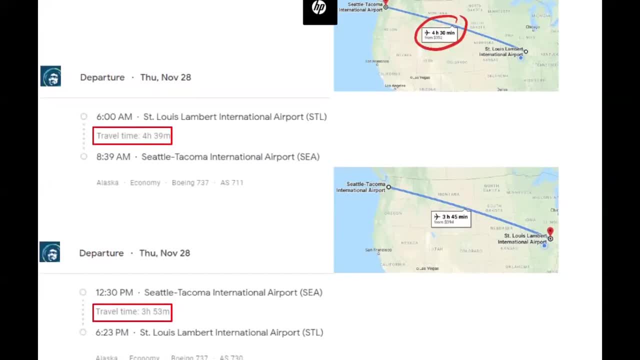 Okay, But if you're trying to fly back from Seattle to St Louis, you can see time is shorter: around three hours and 45 minutes. Okay, Also find this information from here. So what is causing this different time For each direction here? 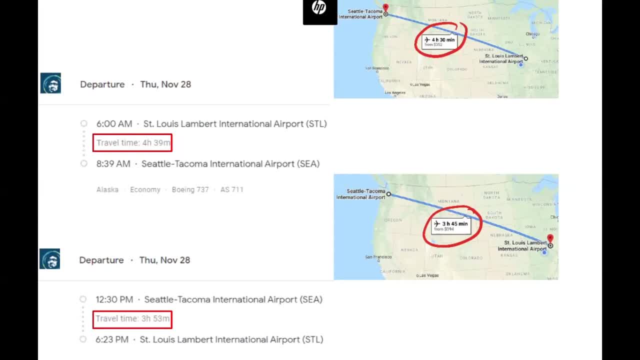 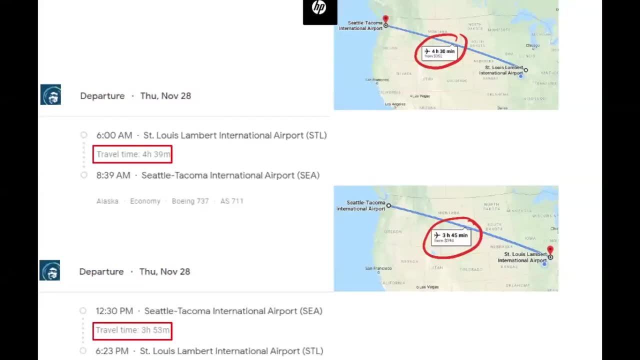 It's also because of the general wind pattern. Okay, So if you think back the wind direction in the mid latitude or in the US- Right, We mentioned that the wind direction is going this way, Right? So what that means is the aircraft can just sit on this wind here when it flies back to St Louis. 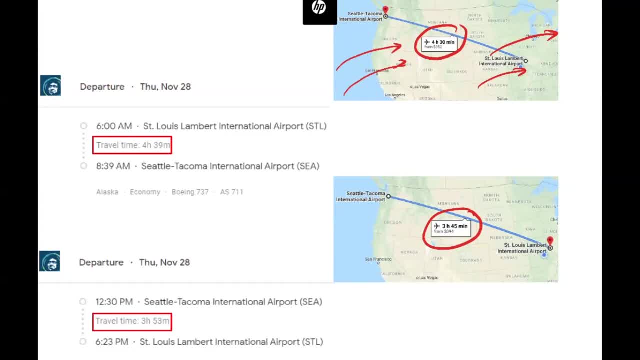 It's not going to cost a lot of fuel, Right? And then we just need a little bit of power so that the wind can just blow the aircraft back to the east Right. And when we're flying from St Louis to Seattle, we have to basically fly against the wind. 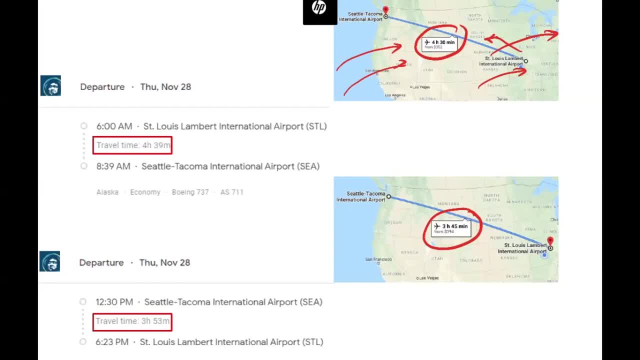 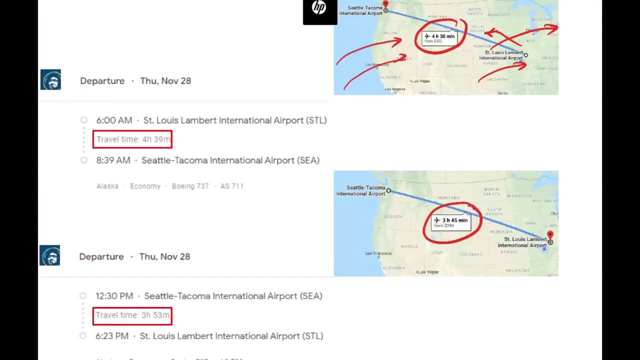 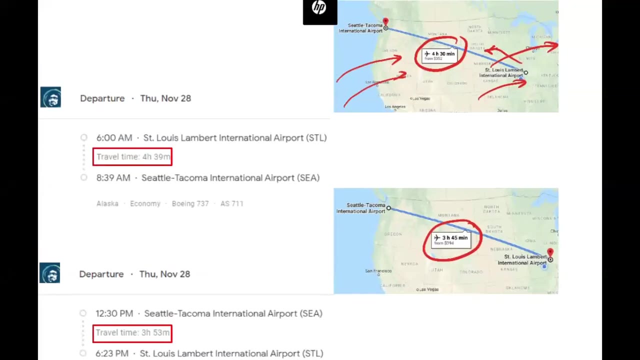 And that is going to take us a longer time. So this happens for the domestic flights And if you're interested, you can also search for the flights going to Europe or going to Asia- And basically this general wind pattern is going to cause a much larger difference in terms of the flight time. 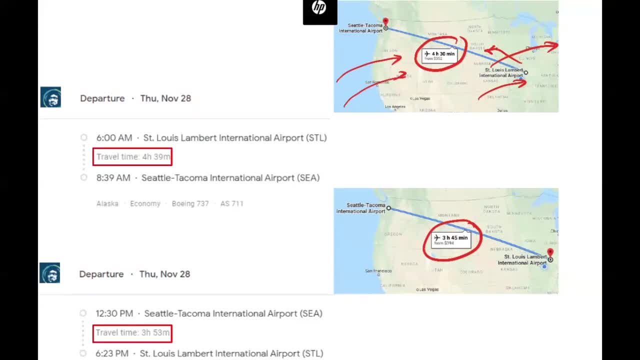 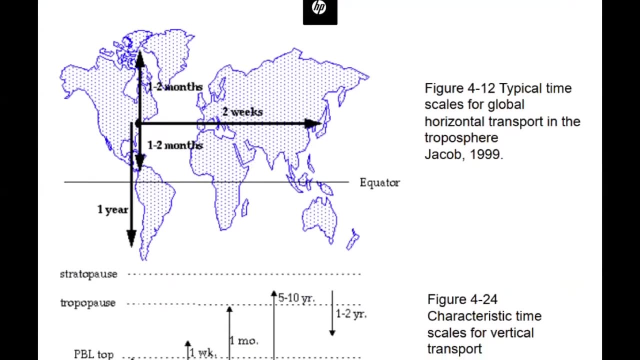 Okay, And this is also caused by the Coriolis force. So why is that important? As I mentioned, the global wind pattern is going to affect a lot about the transport of the air pollutants. I mentioned that We're assuming that we're trying to build. 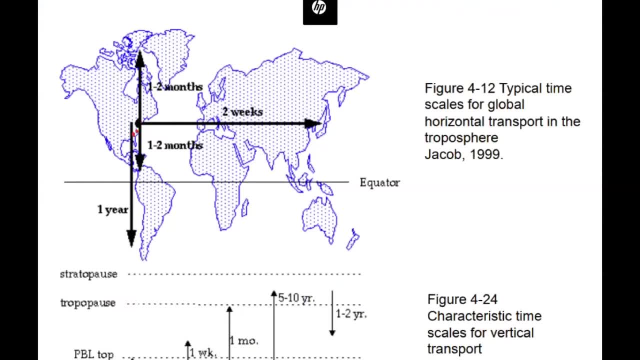 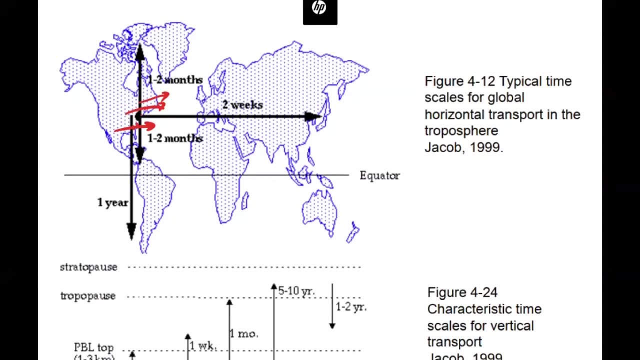 Nuclear power plants. Right, We want to build those nuclear power plants at the east coast, mainly because the wind is going to go this way at the mid latitude, Okay, And it is going to affect a lot of these, These air pollutant transport scenarios. 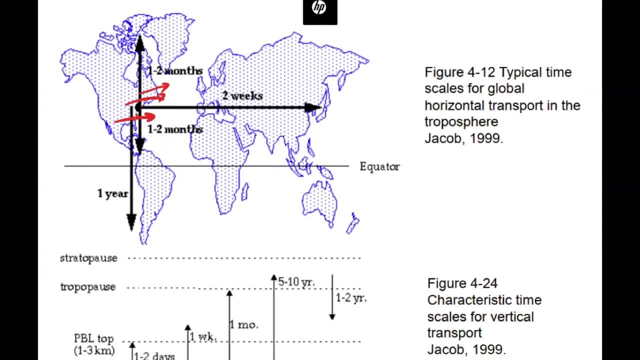 So, for example, if you're trying to understand the transport of the air pollutants from west to east, at the mid latitude, It generally just need two weeks for the pollutants to transport from the North America to Asia. Okay, It is also the same when we're talking about the Fukushima nuclear power plant disaster. 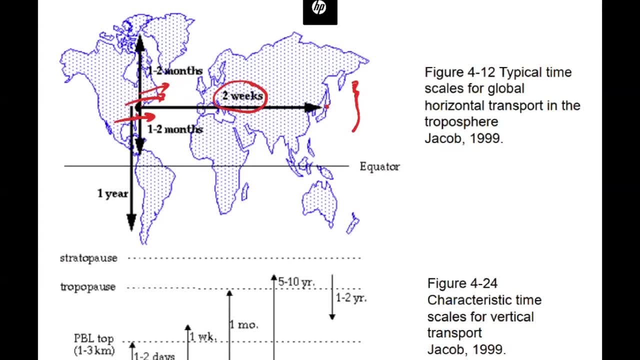 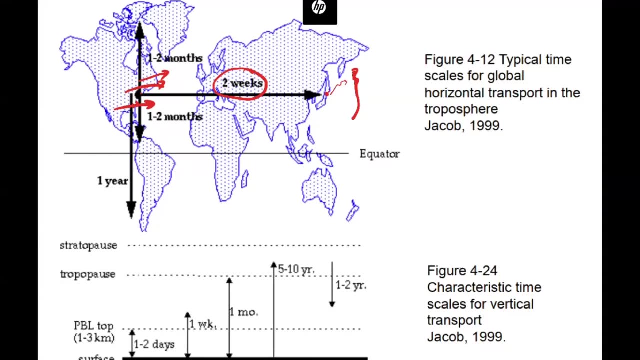 Right When it emits those radioactive particles into the atmosphere. It also took around this time for them to transport to the North America And then you can also notice that for the air pollutants to travel from one cell to the other, We mentioned that we have different, three different cells right at the equator. 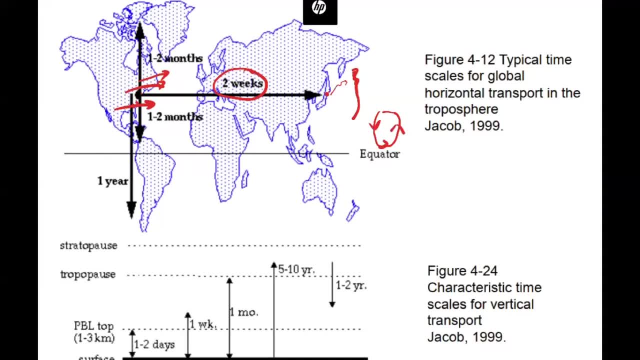 We have this Hadley cell Right And the at the mid latitude we have this Pharrell cell And then at the polar region you have the polar cell. Okay, So in each cell the transport is quite efficient. For example, in the mid latitude you just need two weeks to transport the pollutants. 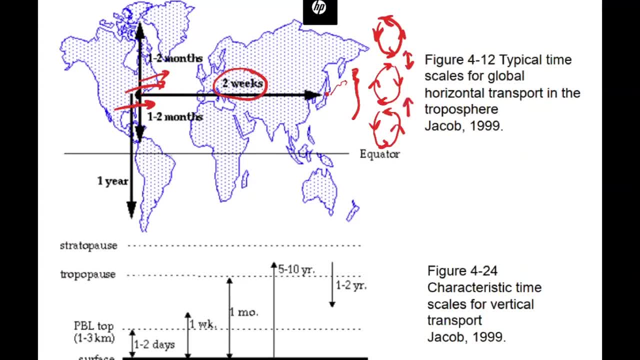 But if we're talking about the transport of the air pollutants across different cells, that's going to take a longer time Around- one to two months- for the air pollutant to transport from the mid latitude, For example, the Pharrell cell, into the polar cell. 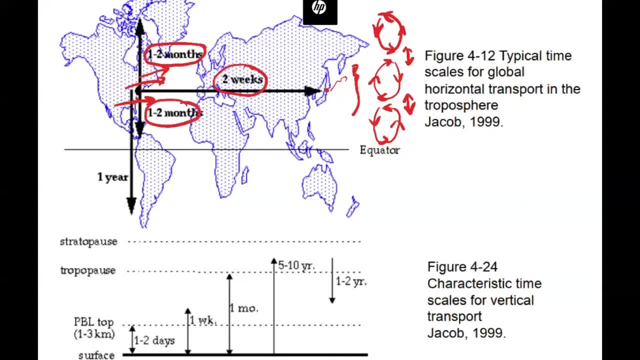 It also needs around one to two months to transport from the mid latitude, So that's going to take a longer time. to transport from the Pharrell cells to Hadley cell, Okay. And if we further want to consider transport across hemispheres, let's say from the northern hemisphere to southern hemisphere, it's going to take around a year. 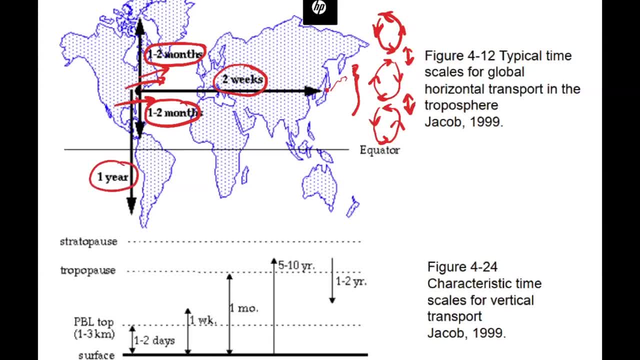 Okay, So in terms of the transport of the air pollutants, it's also going to take a very long time, Right? For example, again if we talk about the radioactive materials emitted here, it's going to take maybe several years To put an impact on the southern hemisphere. 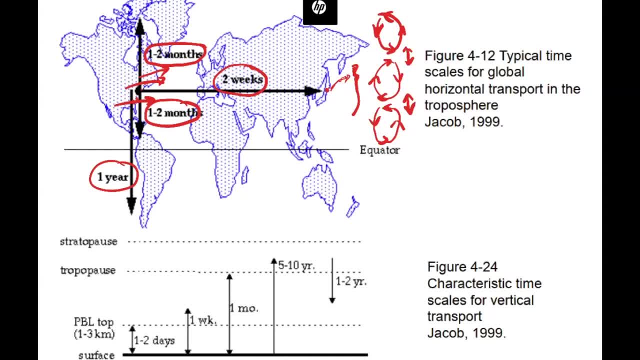 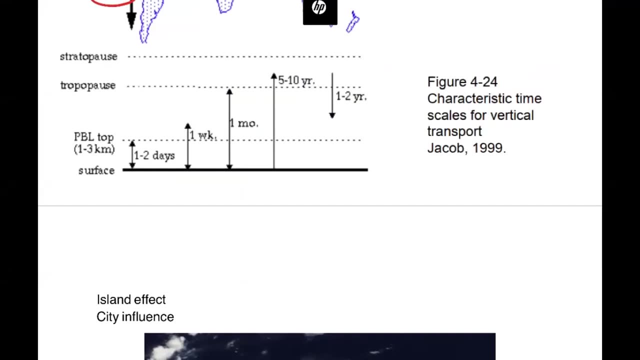 But its impact on the northern hemisphere, especially the mid latitude, is going to be very rapid. Okay, So this is a transport regarding the horizontal direction, And there is also the transport in the vertical direction. Okay, So we can separate our atmosphere into several layers of the air. 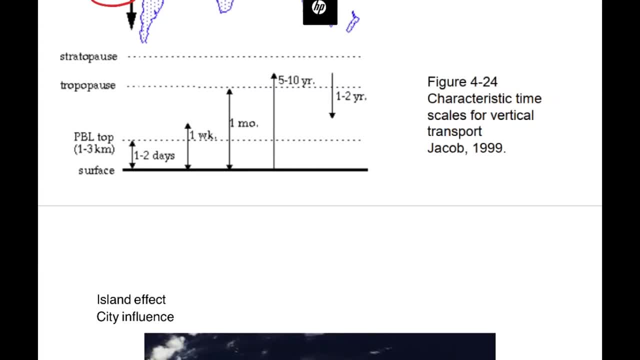 So, if you remember, We mentioned about the troposphere. Basically, the stratopause or the tropopause are just the layer or just the boundary that we mentioned. Okay, So within the boundary we call this as the stratosphere, And then within here we call it as the troposphere. So we mentioned that. I would say Almost all of the human live in the troposphere Right. So I also mentioned that the tropospheric ozone It's a criteria or a pollutant, But the ozone in the stratosphere is beneficial to human. 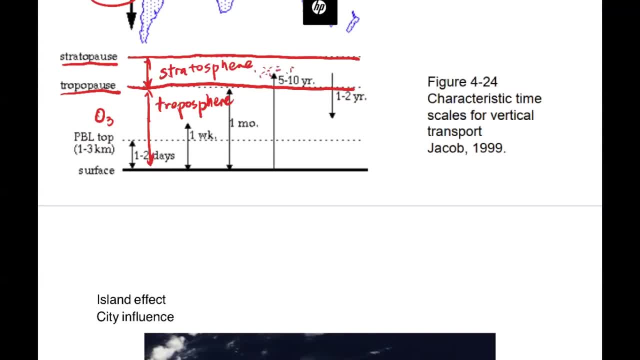 Right, Also here, It's going to block the UV radiation. Okay, We also mentioned that the ozone hole is happening in the stratosphere. Okay, So we have these different layers of the atmosphere And if we talk about the transport, 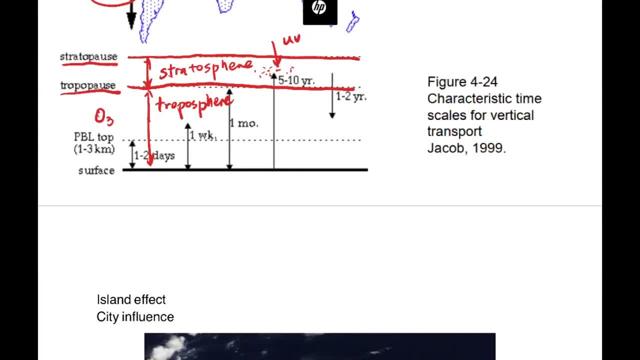 We talk about the transport of the air pollutants Within different layers or within different Layers of atmosphere or across atmosphere. You can see that At the bottom of this troposphere we have this layer called the planetary boundary layer, Or this PBL. 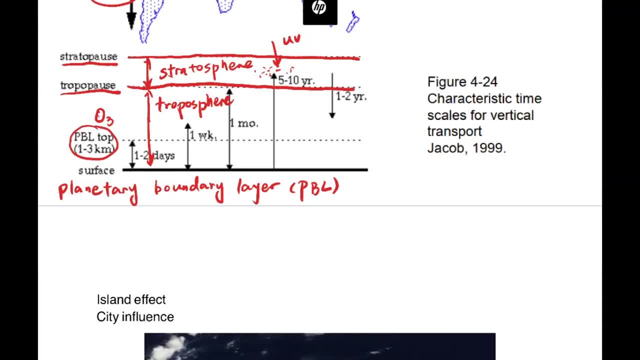 So the planetary boundary layer is Just around one to three kilometers above us, Okay, And the air within this boundary layer mix very well, So it's just take one or two days for the air to mix, Okay. So, for example, we have a coal fire power plant. 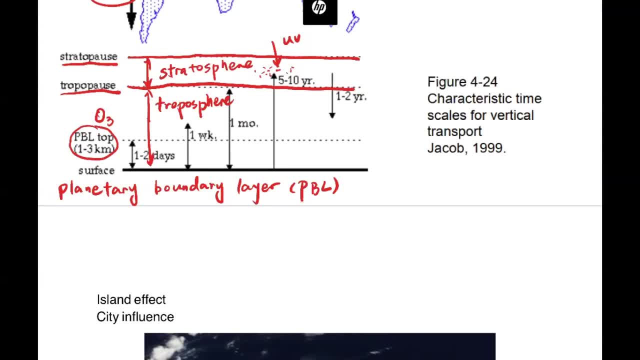 And it's just needs one or two days- one to two days- to Let those pollutant to reach to around one to three kilometers Above us, And this is also the location where we form Clouds. Okay, A lot of clouds are being formed. At this planetary boundary layer And it normally takes around a week For the pollutant to penetrate the boundary layer to Further Penetrate into the lower troposphere. Okay, And takes around a month for the air pollutant to reach to the. Top of the troposphere, And if we talk about the transport of the air pollutants across the Tropopause, Then it's going to take around five to 10 years, Okay, And similarly for the, For the component of the air to transport downwards. 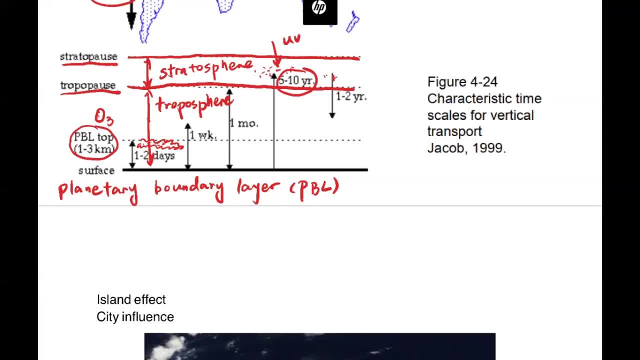 Go across this tropopause from the stratosphere Towards the troposphere. It also took around one to two years. So that's why we're very concerned about the ozone hole Right. So we mentioned about the CFC, Right. We use a lot of these chlorofluorocarbon. 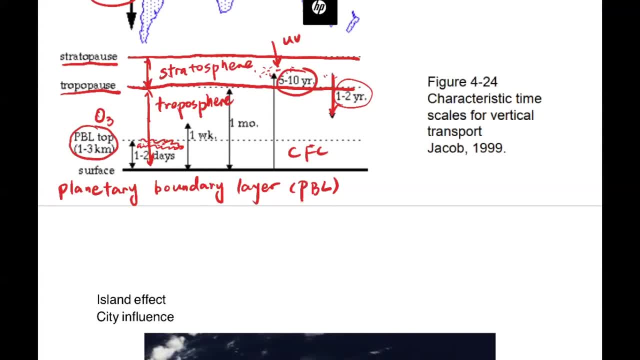 For the refrigerator refrigerators And it's causing the ozone hole. But the transport of these species Actually takes years to penetrate Into the strat, into the stratosphere Right. It's highly likely that a lot of these CFC, which are very stable, 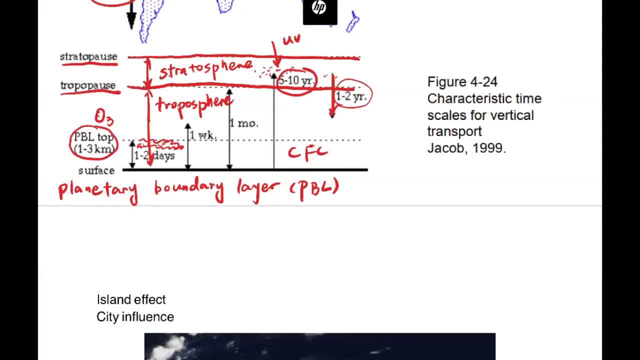 In the atmosphere are still staying in the Tropopause They haven't penetrated Through. They haven't penetrated through this tropopause To To deplete the ozone yet Okay, So if you track the ozone concentration, It might be still decreasing.